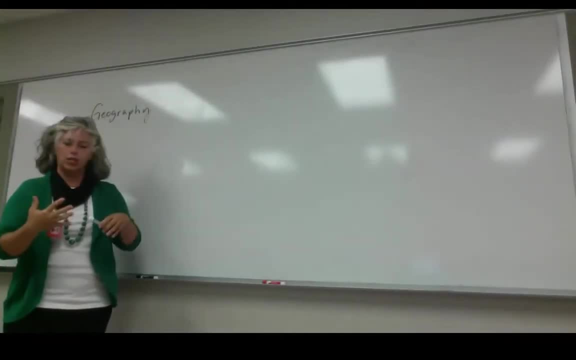 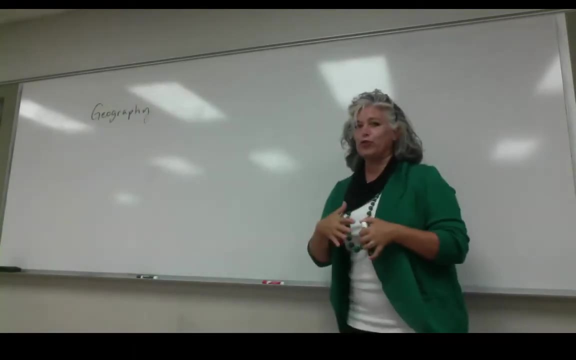 Okay, so this is our first session of geography aside from the syllabus and reaction paper day that we reviewed, And so today we're going to get our first bit of notes. Y'all, please help me remember that this clock in the room is not right. Like how far into 10 o'clock. 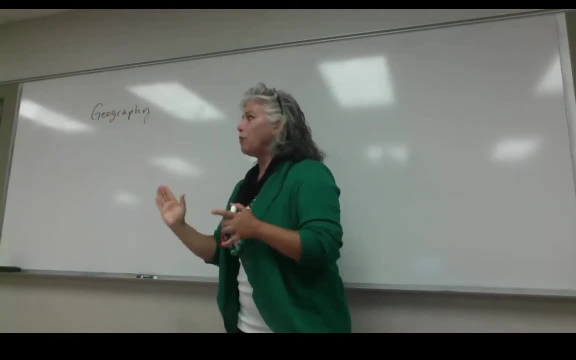 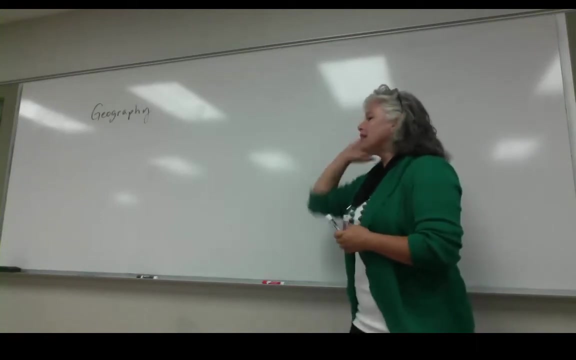 are we already 10.07.. Okay, please help me remember to stop at 10.50, because I'm not used to this shorter time format, I'm used to the hour and 15 minutes. So please help me stop. you know, flag me down if I'm rattling on. Okay, so let's talk about what this class. 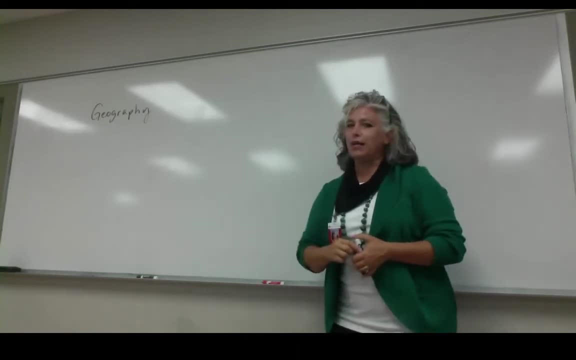 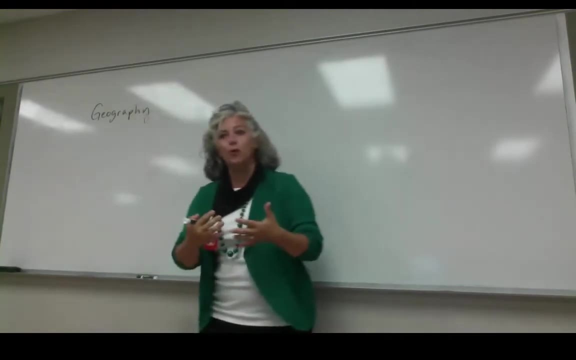 is and why you're here. This is one of the social science electives that's on most people's general education degree plan. So this is counting toward your general education degree plan as electives, usually for wherever you're going to transfer as electives here for our 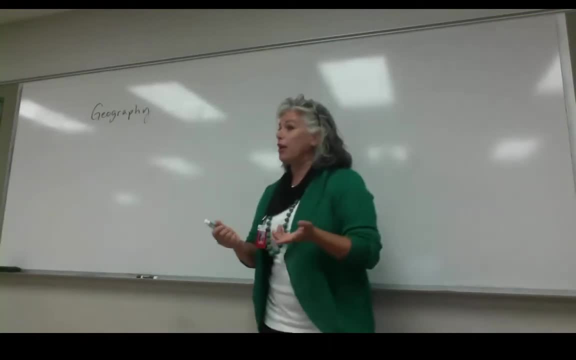 associate of arts and associate science degrees. Additionally, are any of y'all culinary students? I know I have a lot of culinary students out there online. so, hi, culinary students. This class: cultural geography, physical geography- the classes that we offer here in geography. 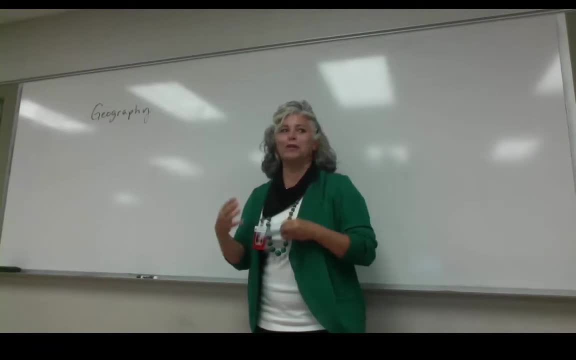 at UAPTC are really great for food related degrees, and it's one of the three. There's only three choices for social science that you can get on your culinary degree, and this is one of them, Because geography, of course, has a lot to. 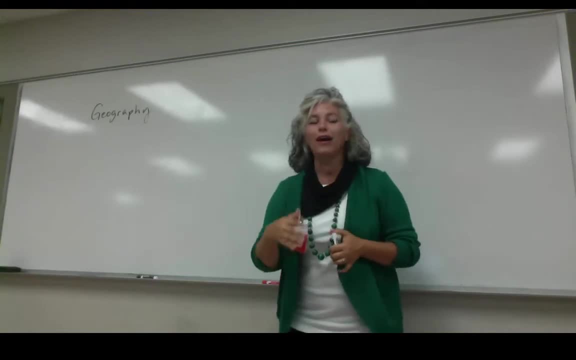 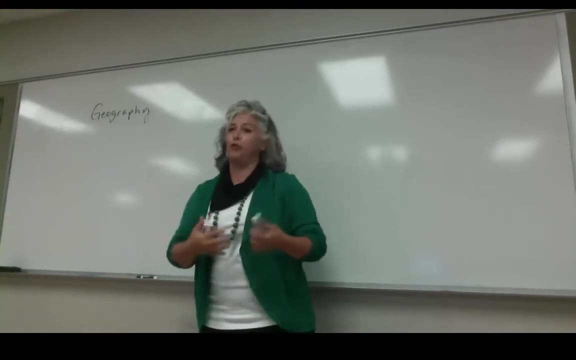 do with the kinds of foods that are available in nature where you are and also the way you're going to be able to manipulate the natural setting where you are in order to produce the food that you need for the population size, for the cultural habits and that kind. 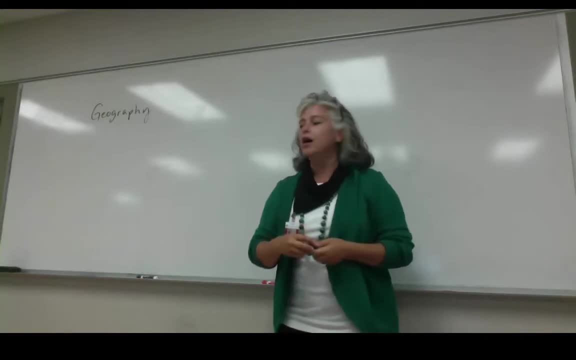 of thing of the people who live there. Okay so, and Ken Lipsmeyer, for instance, he's the wine and spirits guy over in the culinary school. He is majorly into geology and geography, and whenever we get to the end of the semester he's going to be like, oh, I'm going to do. 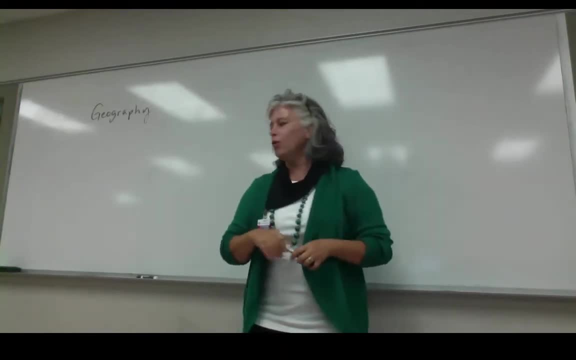 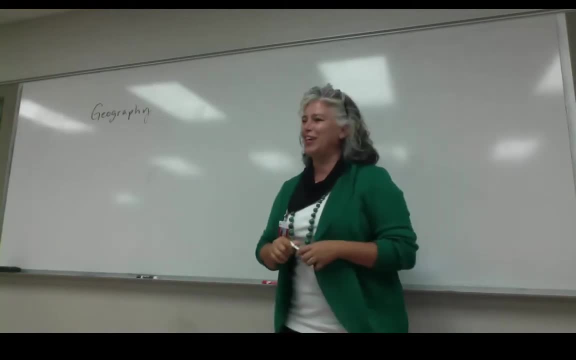 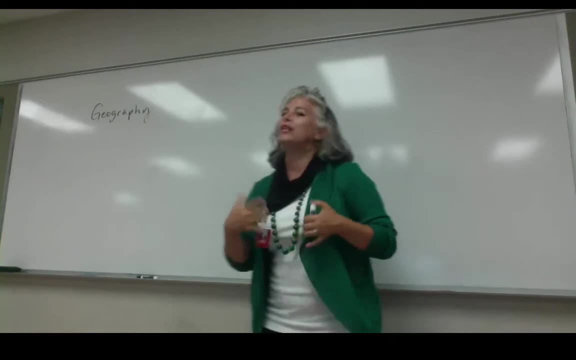 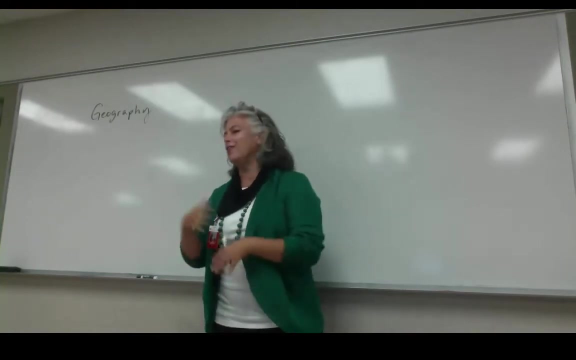 we're just like two geeks in a peapod together about geography. So anyway, it has a lot to do with a lot of degree plans and a lot of general interests, that whether you're going to go into social work or law or nursing or culinary or welding or anything in between. 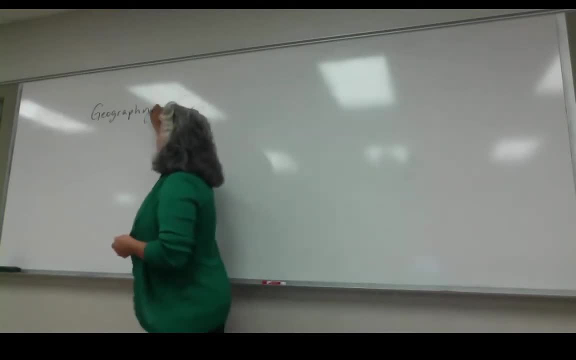 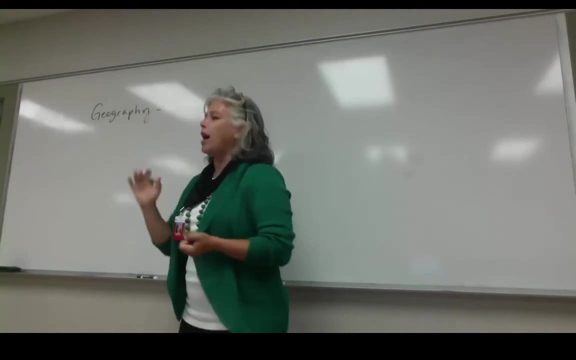 this is a human science. We're going to define this word or get some key terms for what geography means here in just a second. I'm not. I don't usually- for those of you who've had me in sociology class before, I usually don't write really. 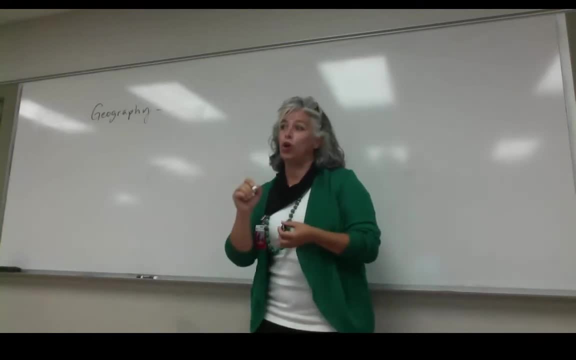 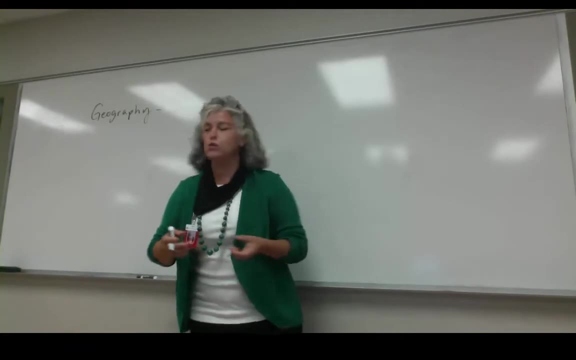 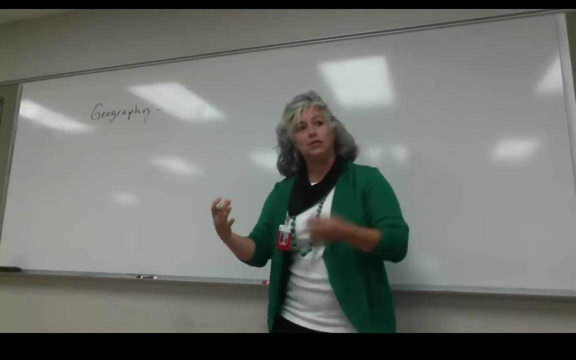 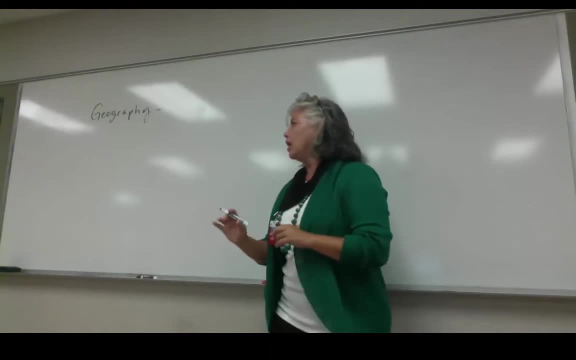 and talk about stuff that you might not know about. So I'm going to stop and talk about some of the stuff down that we talk about. But usually when I, you know, give you a key vocabulary word, a pretty important one like this one, I don't give you a sentence long. 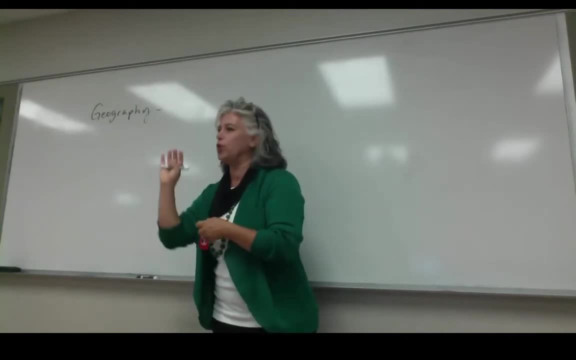 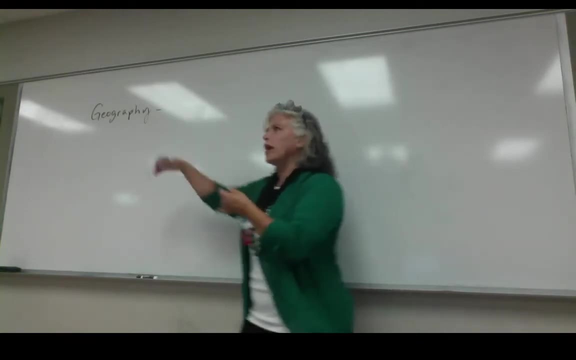 definition. I give you key words that you need to put in your own unique sentence to define the word. Okay, So I was about to write human geography on the board also, but let's go ahead now and give you those key words that go into the word geography. Okay, Go. 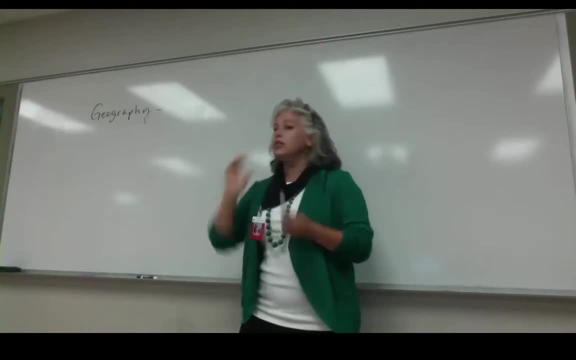 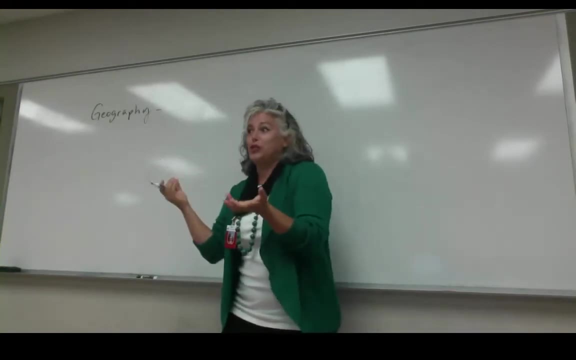 into the definition for the word geography. So literally the word geography means drawing the world, drawing the earth. Geo means earth and graphy is drawing of some sort. A biography is sketching out somebody's life. Right, Geography is sketching out the landscape. 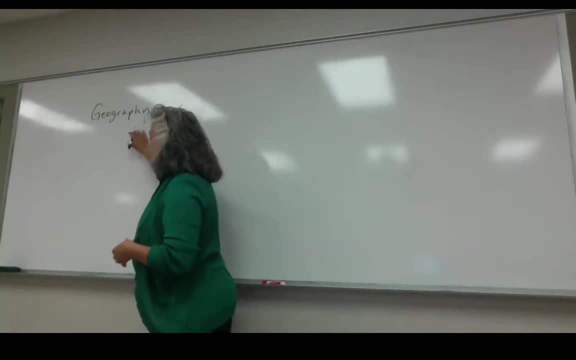 Sketching out the world. The key terms- I'll wait just a second because I see some folks writing that down- The key terms that you need to know for a good definition of geography. Geography is about space. I don't mean outer space, I mean things like these: six foot distancing. 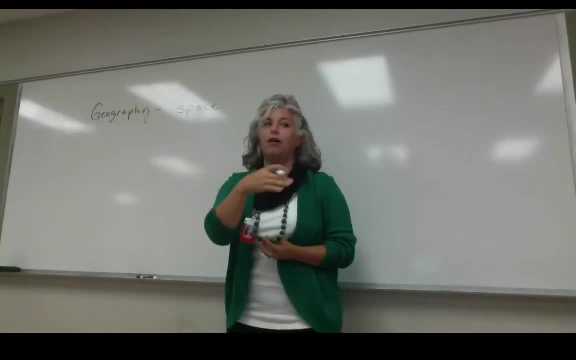 signs that we're following, following up, observing that six foot social distance right now Space. It can be this micro level or it can be like the general shape of the area of Arkansas. that pretty much all of us. when I say that Arkansas do you. can, you like, see it in your 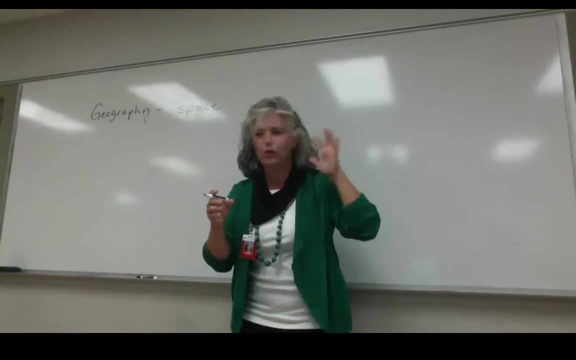 head. You've seen it enough, at least on the local weather reports, that you kind of know the shape of the state. We maybe know the shape of the general shape of Alaska or the United States in general. Right, So the space is, space is always something that has to. 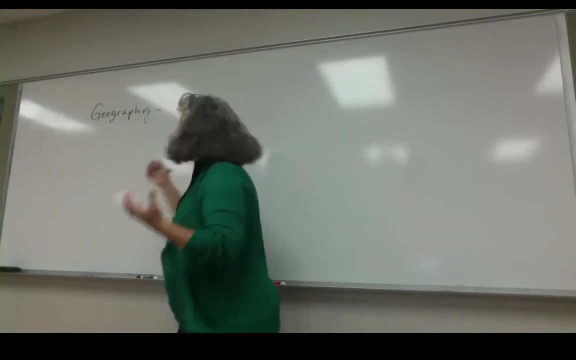 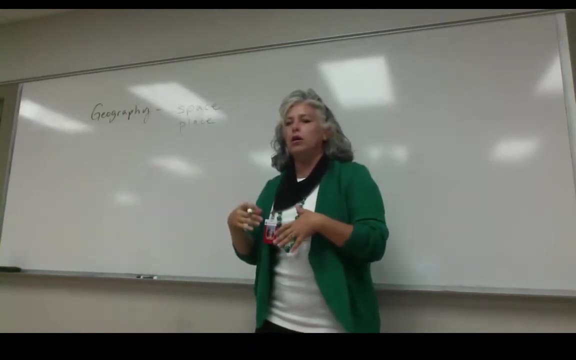 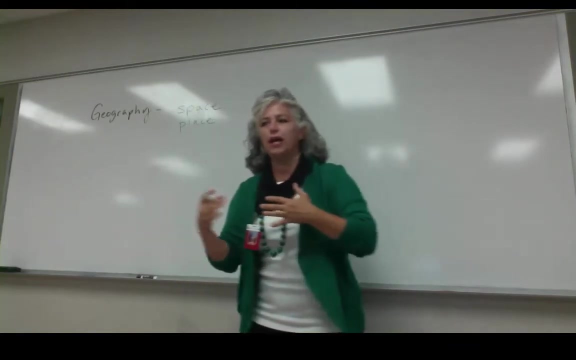 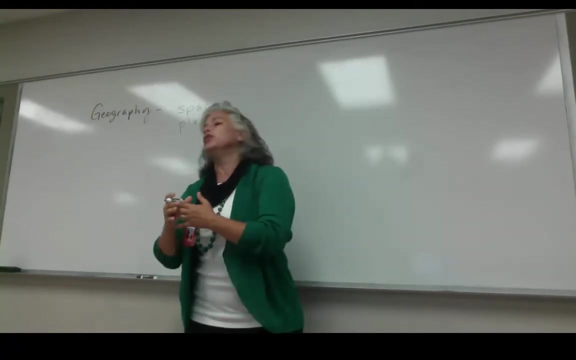 be in a good definition of geography, because it's the way we understand space. It's the way we understand place, Some so. for instance, we have a river market district in Little Rock. I used to take a whole bunch of students When I teach cultural anthropology, I take students sometimes as a field trip to 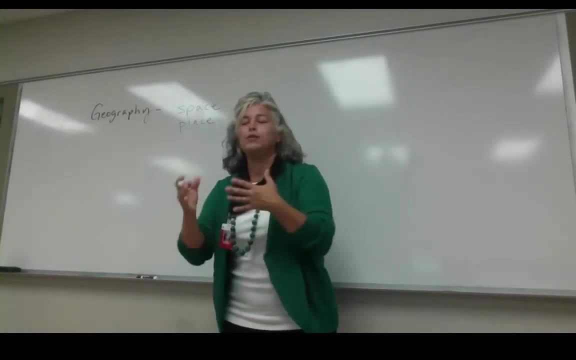 some archaeology lectures that happen once a week, once a month, sorry, In the river market. I have a bunch of students that go to the river market. There's a presentation room in the nature center there and that's the place. the river market, the presentation room at the Wood-Stevens Nature Center, That's the place where we go and do. 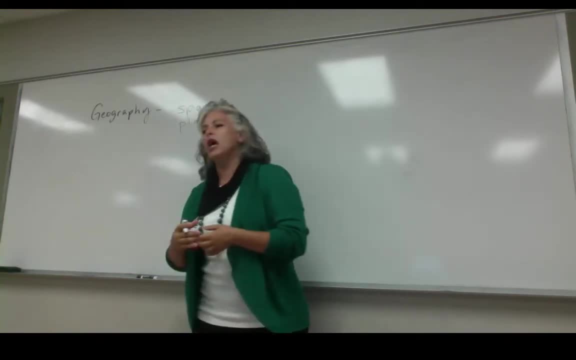 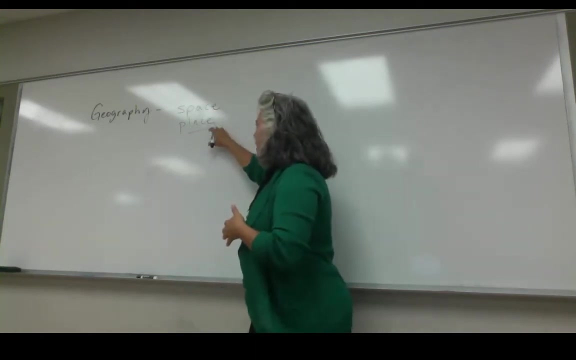 these geography- excuse me, archaeology- lectures. Some of my students over the years have been afraid to go to river market district- the place at night- because it's in the big city of Little Rock And Little Rock's scary to some people. So this is a mental scape: This space and this place, these things- here's some more key terms. these things actually exist in the physical environment, but they actually exist too in our mental scapes. 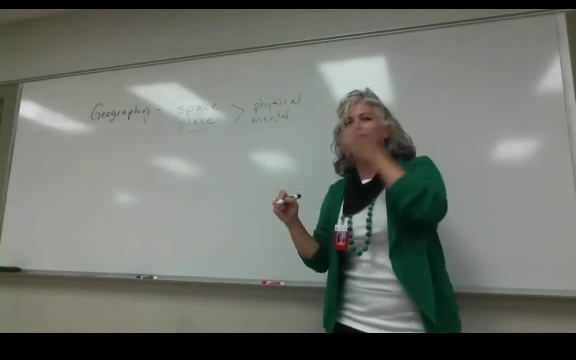 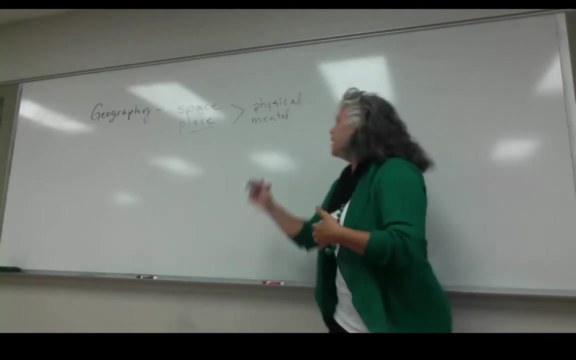 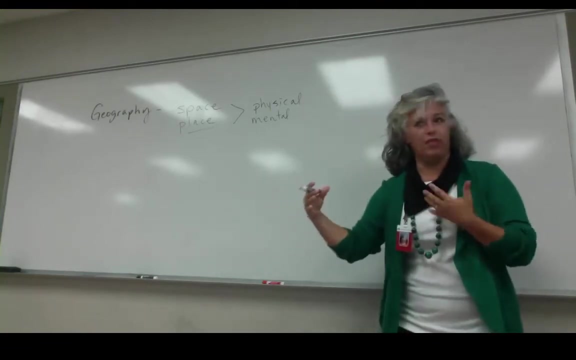 We have ideas that define space and place. So they are physical things like six feet is a physical distance we can measure. but mentally, the six foot right now is for our safety, it's for our comfort, It gives us a general confidence in being here together right now because we're going to observe that space right. 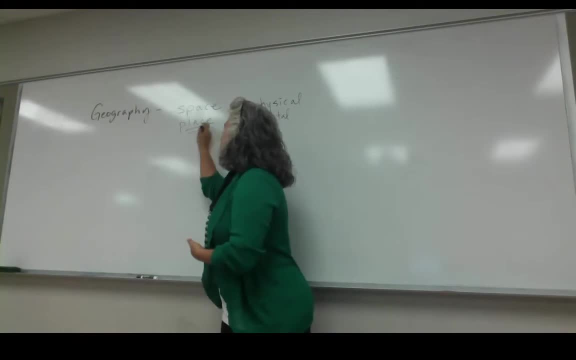 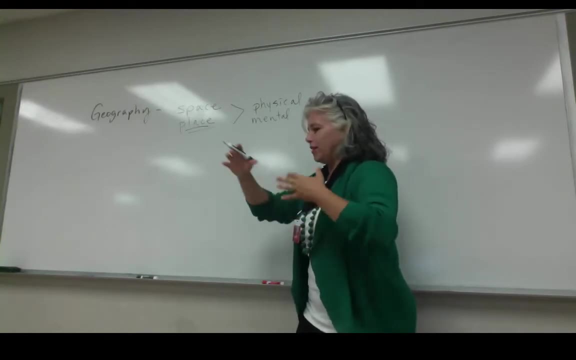 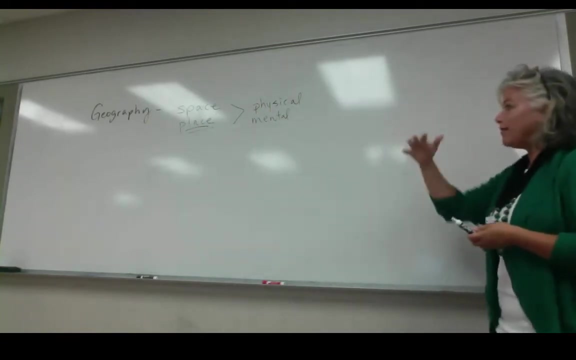 I have, you know, lots of examples of place That are, in general, large geographic features, like the Rocky Mountains or the Mississippi River is. there's lots of space and places along the Mississippi River right as it runs through the geographic United States. 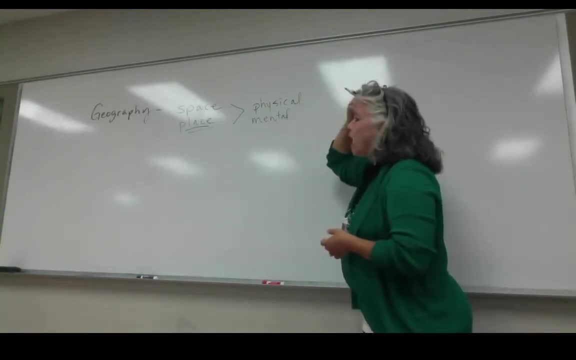 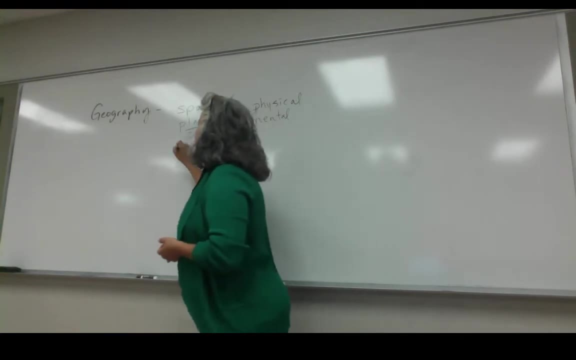 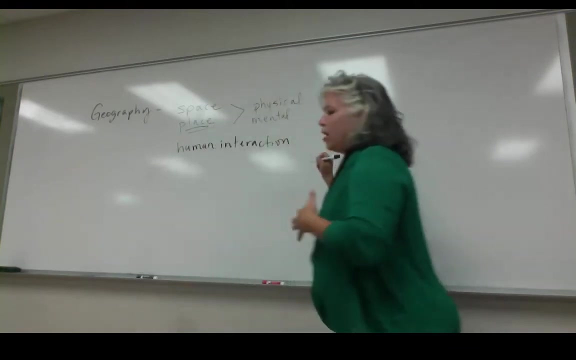 There's physical aspects of it, there's mental concepts, mental pictures of these things, Other key words that need to be in a good description of geography. So geography has to do with human interaction in that environment. How do humans interact with the space and the place? 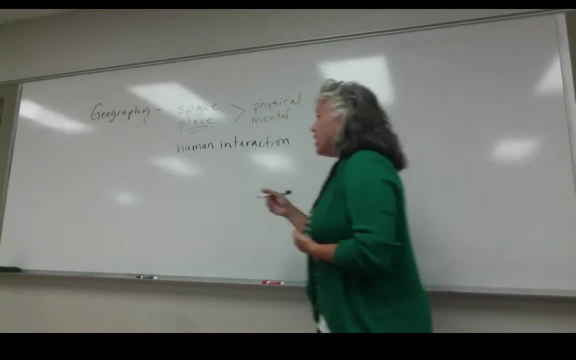 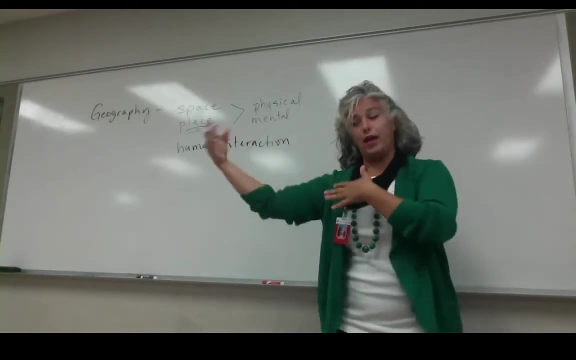 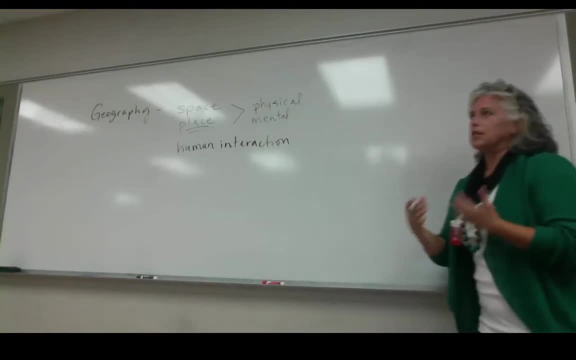 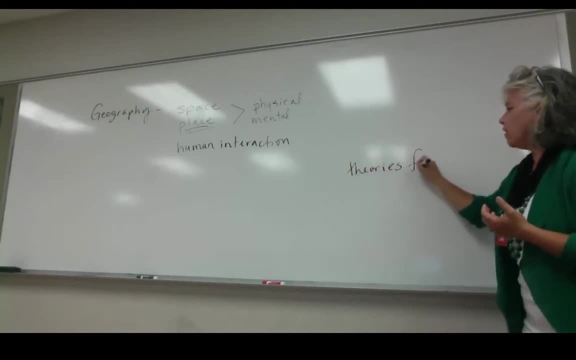 just like theories for explaining why something happens where it happens, So theories for analysis in cultural geography, the old time, or traditional theories. one of them was called environmental determinism. Environmental determinism: Your environment literally determines what your culture is going to be. 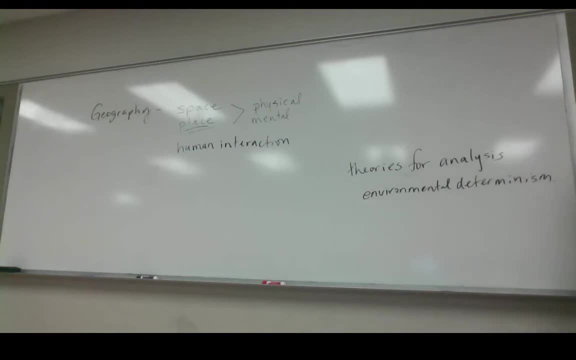 That's the idea behind environmental determinism. For instance, think about what we build houses out of in Arkansas. What are some of the things, the materials, that we use to build houses out of in Arkansas? Not a trick question: Wood bricks. We got tons of clay in the soil in Arkansas, Right down the interstate in Little Town. y'all know what it's called where the brick manufacturer is down close to Malvern. it's called Perla, Right down the interstate here. 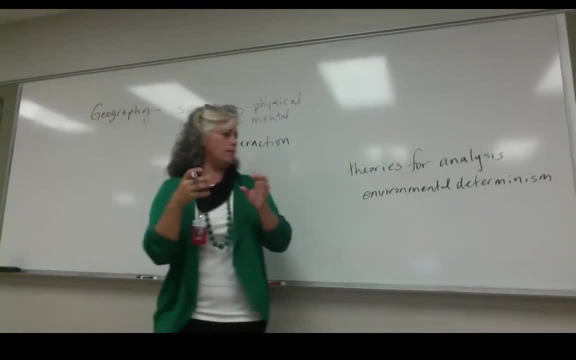 the huge Acme brick manufacturer, because the physical environment has a whole. There's a whole bunch of clay in it. There's a whole bunch of wood up in the Boston mountains around Fayetteville, Arkansas, the Ozarks up around there, What else do you think probably enters? 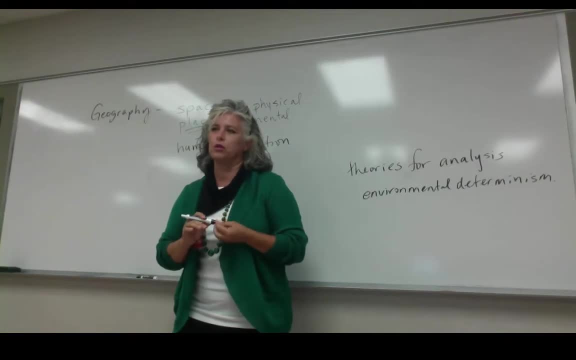 into how they build houses and structures in the mountains Rocks maybe. I've seen a lot of rock houses or rock foundations or rock walls and things like that. So this is one kind of way I'm describing this, because it maybe helps you understand what environmental 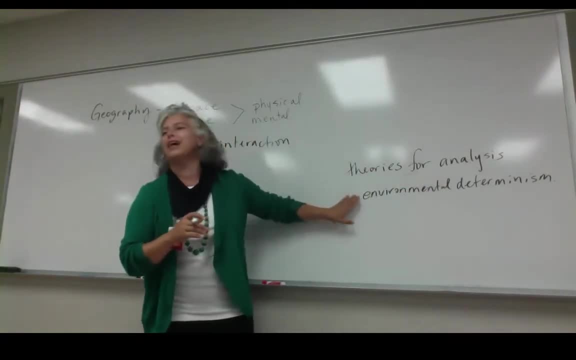 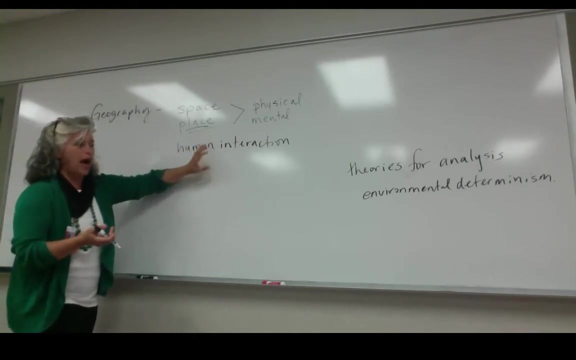 determinism means. Let me emphasize that this is kind of an old-fashioned way of thinking in geography. We don't really use environmental determinism very much anymore. Human interaction with the environment is very, very important. However, we're very, very creative and if we want, 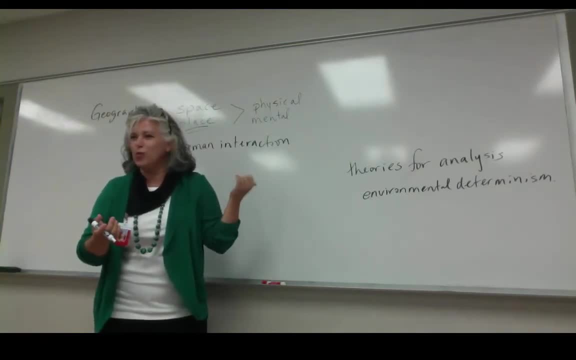 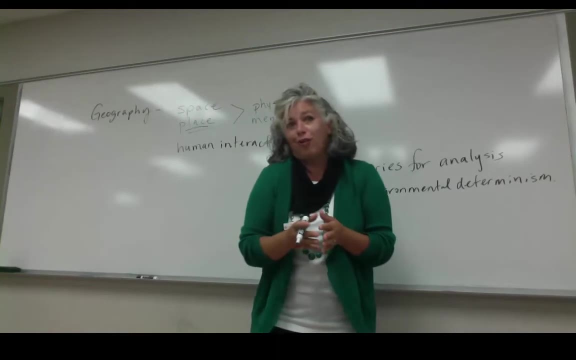 to do something in a place where it's not possible. what do humans tend to do? We tend to figure out a way to make it happen. Humans can't fly Right, But can we fly? Yes, we figured out a way to make it happen right. We built a machine that enabled us to do it. Now we're building other machines that enable us to do it. We used to just be able to fly around the earth, and now you've got what's that company? Virgin Galactic- is that what it's called- that sends people. 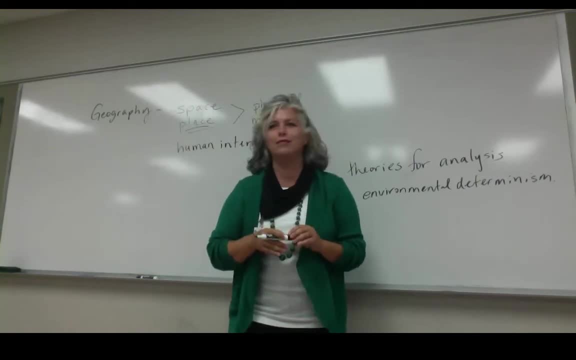 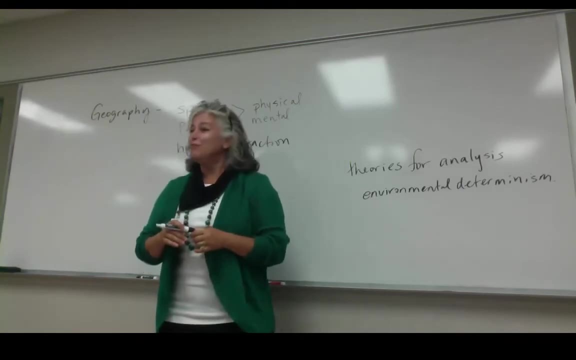 or what's the Tesla one that's sending people in orbit in outer space, right, Like we can do that now, just as civilians. Well, you can, I'm going to stay put, But right, it's possible to do a whole bunch of things. 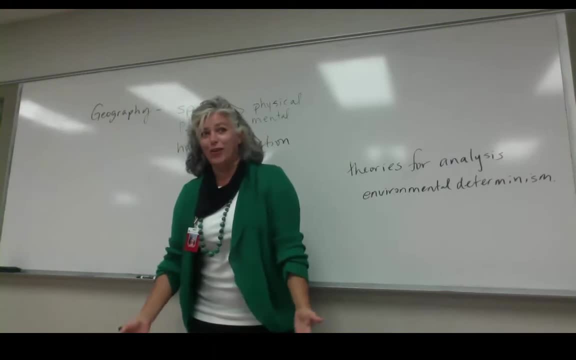 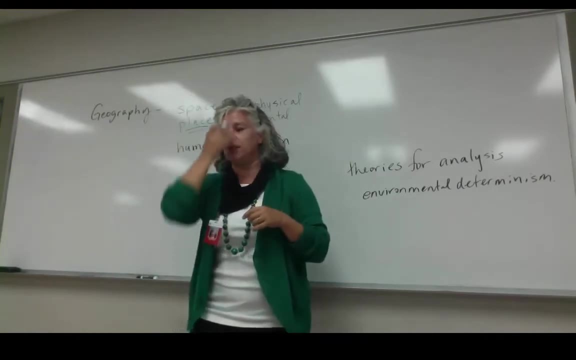 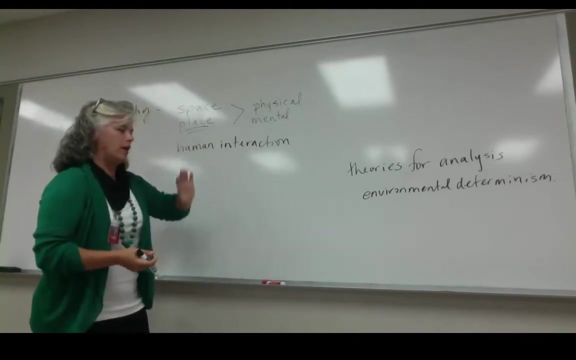 that our environment, like gravity, keeps you on the ground, but it's possible for us to build something that helps us move in the ways that we imagine are possible. So environmental determinism is kind of like the history of where geography was when we first started. 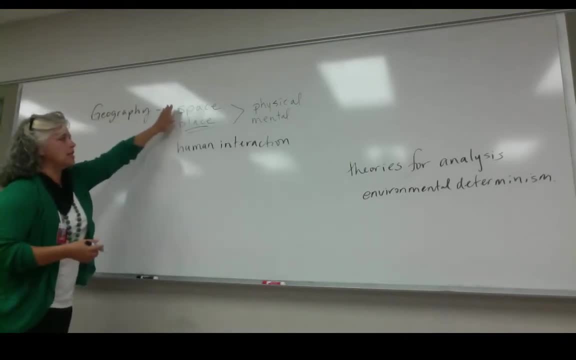 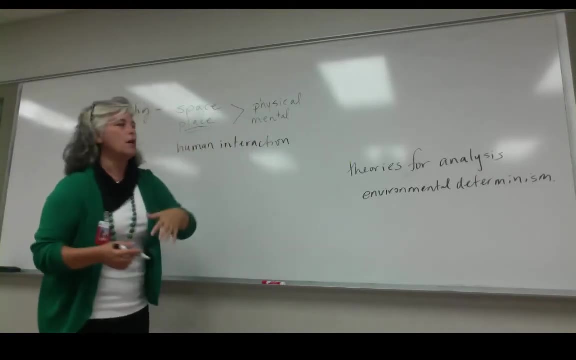 with this social science of trying to understand space and place in our, in the physical space, In the physical sense, but also in our minds, and how we create mental scapes of our space and place and the human interaction that we have with our environment. 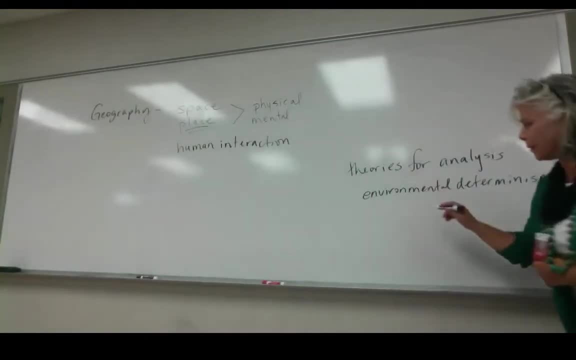 So environmental determinism? it's a way for understanding our space and place that proceeds with the assumption that whatever is in your natural environment determines, it, sets the stage for what your culture is going to be like. We don't really say that this is entirely 100% valid anymore. 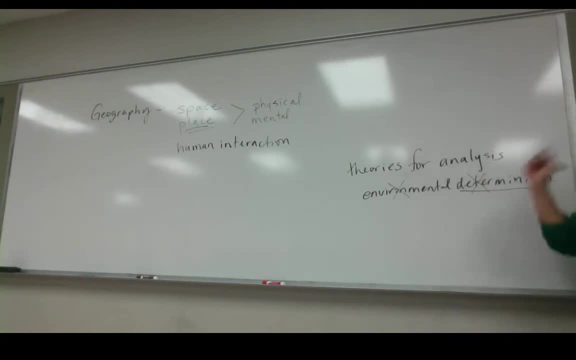 There's some really good arguments in environmental determinism. However, what we use most often now is something called possibleism. Just stick an ism on the end of it and it can be a theory for analysis If something is, if we can imagine something like flying and defying gravity. 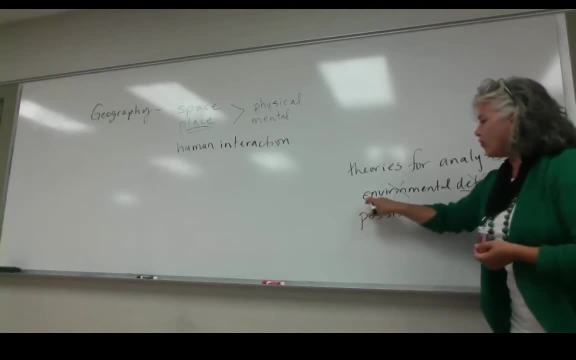 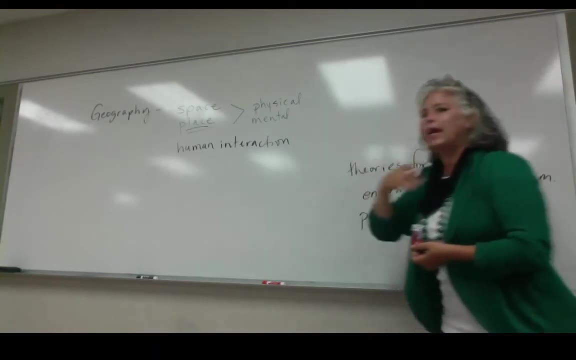 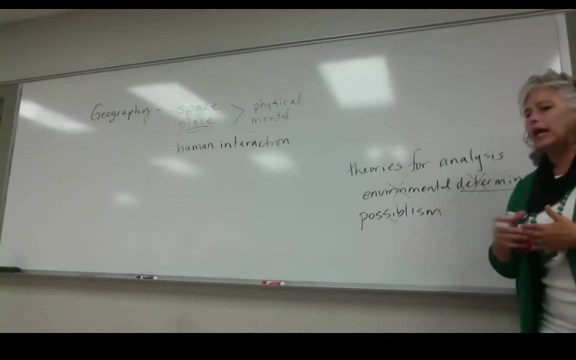 in that way, then we can overcome the physical constraints of our environment and whatever we mentally imagine can happen, we can figure out a way to make it possible. And this is usually the attitude that most geographers, as social scientists, have today is that, if you can imagine it, 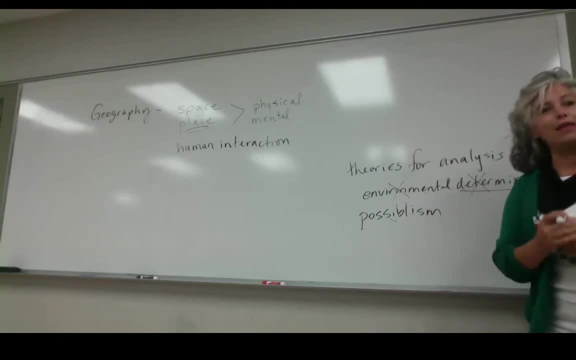 it's possible. we just have to work hard enough to get it. I might not get it in my life, I might not get it in my lifetime, but maybe grandbabies will figure it out in their lifetime. Have you all seen the movie The Martian? with what's his name? 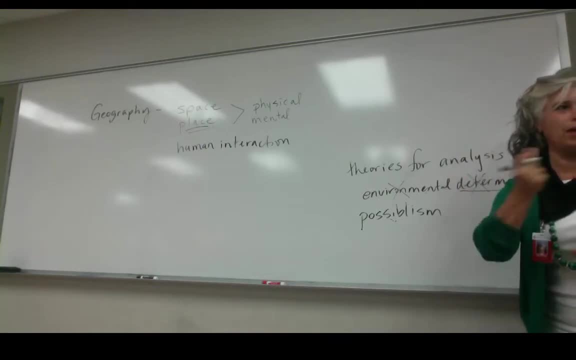 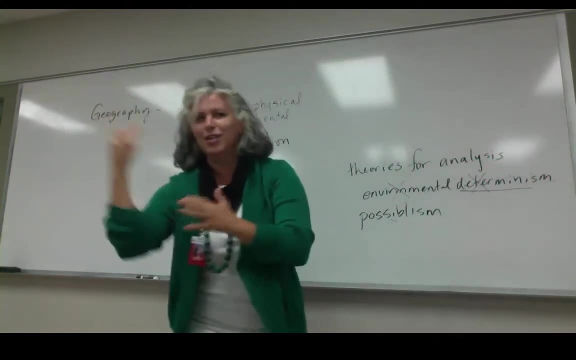 What's his name? It doesn't matter, Siri could tell me, But anyway, Matt Damon, Matt Damon, thank you. Yes, we subliminally. she shot that message to me over space and time. Okay, so The Martian? what is it? 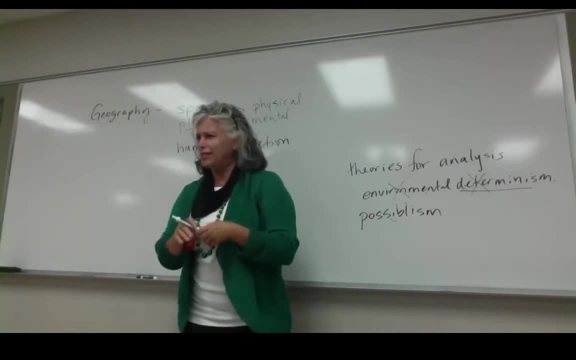 He's left behind accidentally. He's left behind accidentally on a trip. He's left behind on a trip to Mars. Why do you think they thought that he died and they left. They thought that he died, they left. he was not dead. 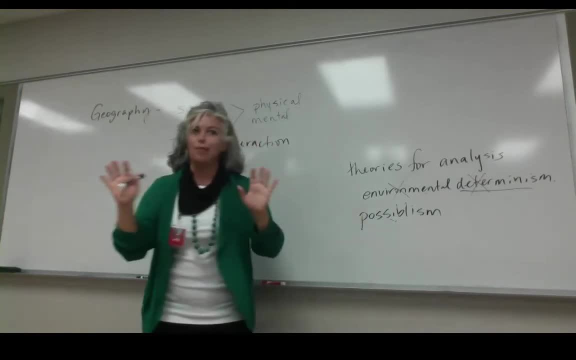 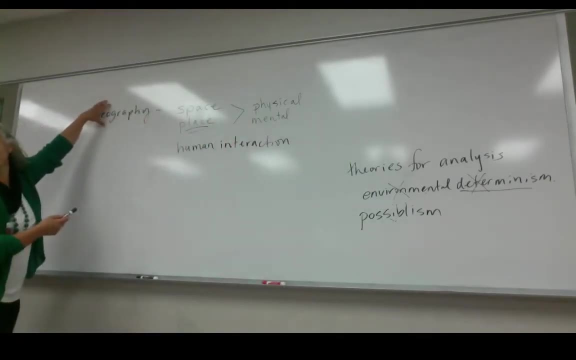 And the environment on Mars. I'm using this. I promise this is a geography lesson here, even though when we talk about geography, this means the Earth. right, Geo means Earth. But let's talk about Mars for just a second. 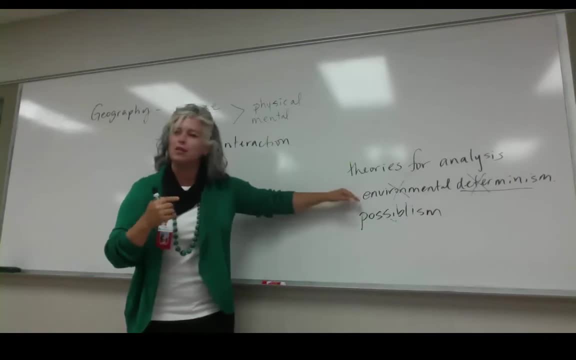 If you used the idea that environmental determinism was really the only way you could analyze the way culture is created, the way humans create culture in the place and space where we exist, then Matt Damon would be dead and we would not have that movie right. 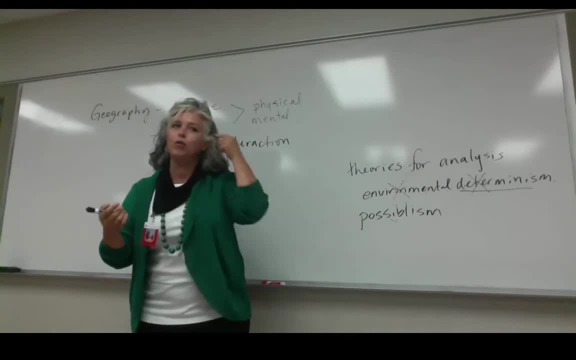 But possibleism is the fact that human beings can figure stuff out, especially when your life is on the line, And that was- or when your culture or your way of life is on the line, And so this concept, possibleism, is the whole thing. 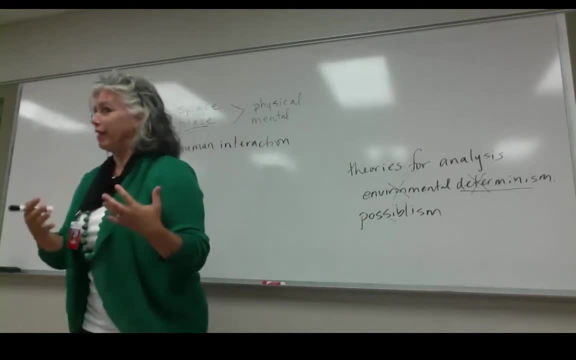 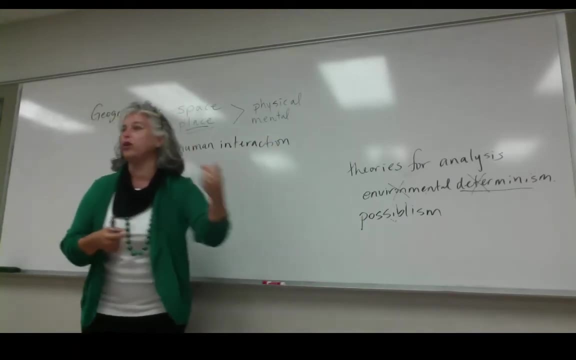 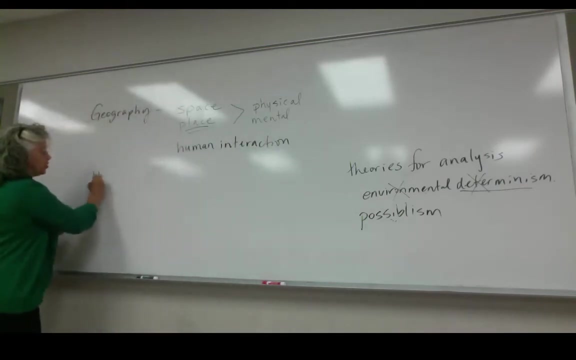 Now granted, yes, that is a fiction movie, but I'm using it as an example because, as we can figure out how to make stuff work on our behalf, And therefore most geographers these days, most human geographers, human geography is the name, it's not the name of our class. 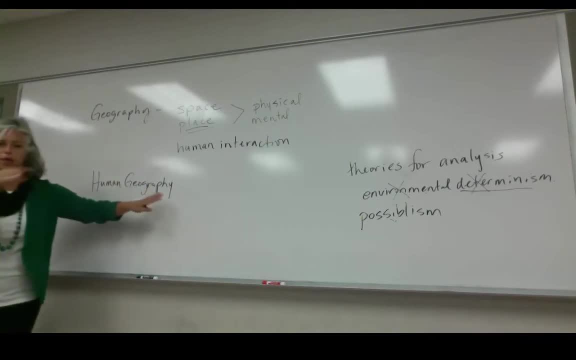 it's the name of our textbook. Human geography is something I can't forget- what the colon is after there. But our class is cultural geography, human geography. They mean the same thing. So cultural geography is the name of our class, Human geography the name of our textbook. 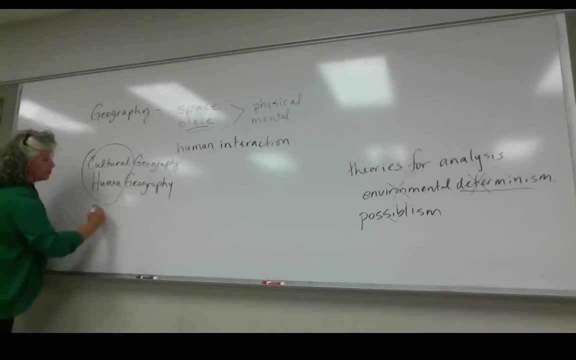 They mean the same thing. This is about behaviors. Behaviors, attitudes, traditions, ways of life, all that focus on the space and the place where we exist, And that's what I'm talking about, Where we happen to be. It's about behaviors. 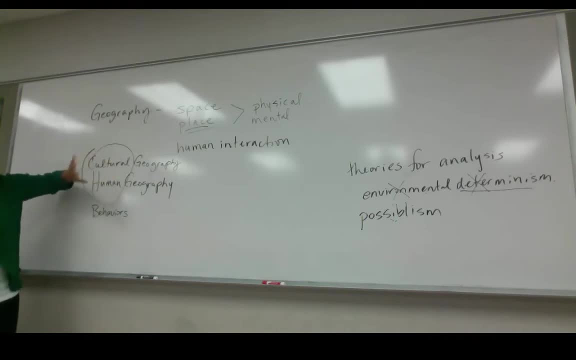 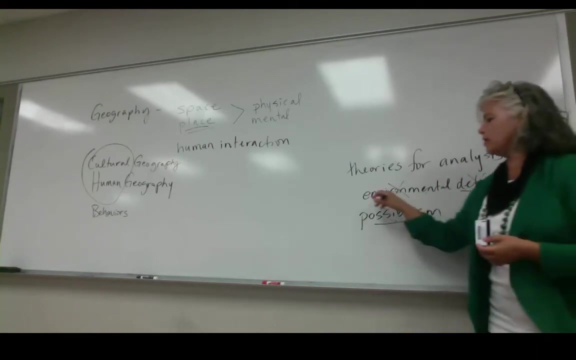 It's the you and me aspect that we overlap with drawing the earth, Geography, Literally. how do we create lifestyles, ways of life around us? And possibleism is really the attitude that we are going to proceed with in this class. We'll talk about some examples of environmental determinism and then also possibleism in some. 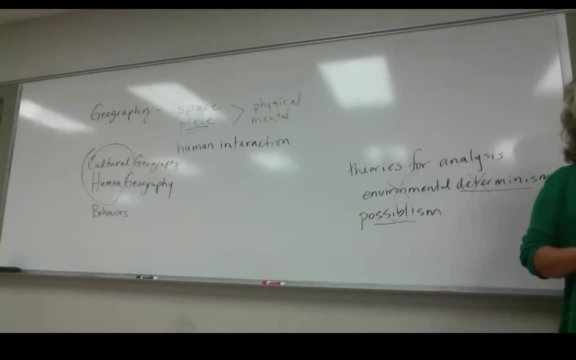 of the things that are planned in science, in medicine, in politics, in colonizing Mars, for instance, which I understand is something that the scientific community, NASA and the international scientific community have a lot of interest in, And so we'll talk about that in a little bit. 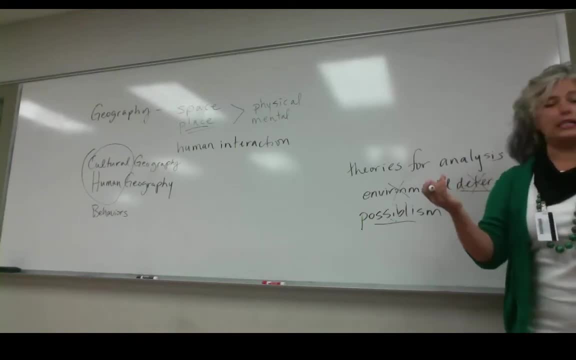 And then we'll talk about some of the things that we're going to pursue. And then we'll talk about some ideas that we're going to pursue and other people who are working on it take extremely seriously. It's not just going to be a science. 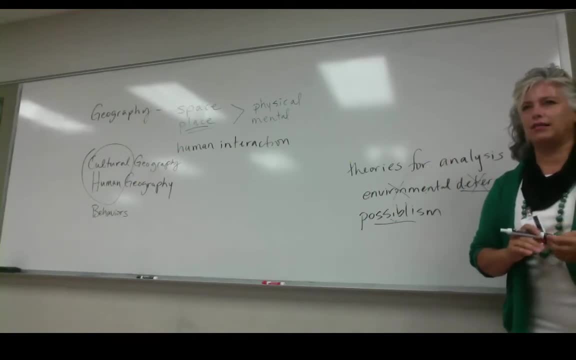 fiction movie. It's going to be, I guess, not colonized. I guess Mars isn't the first one. I think the moon is the first one that they're taking seriously. You know, a colony on the moon? So clearly that's not. 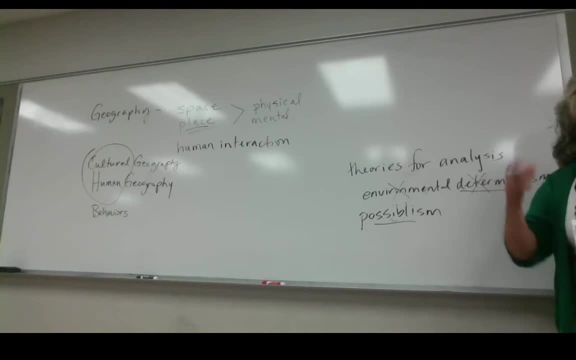 a place where you and I can walk around without assistive devices- Right Oxygen and things like that. So it's going to be interesting to look at some of the ways that we have manipulated. We have not allowed the environment to determine what reality is, but 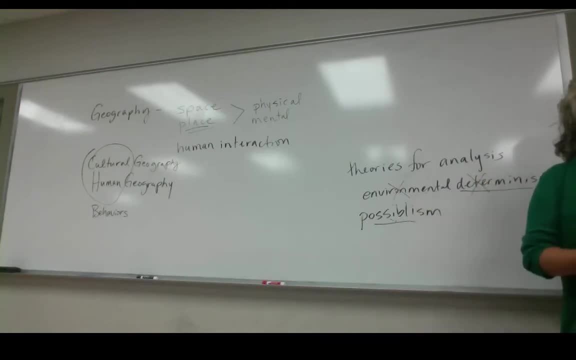 instead manipulated it. so we create reality ourselves in the place where we are. Okay. So there is another keyword that at the beginning of chapter one you'll read about. So we have cultural geography on one side of geography. Let me write that back up here, And that's: 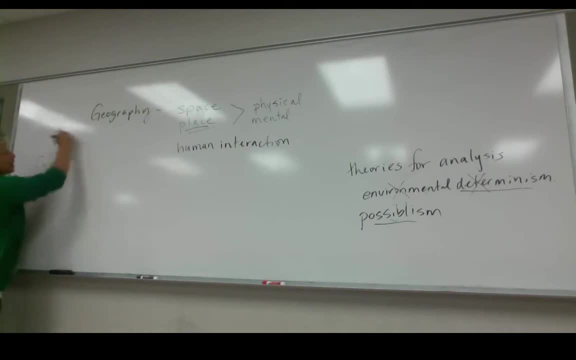 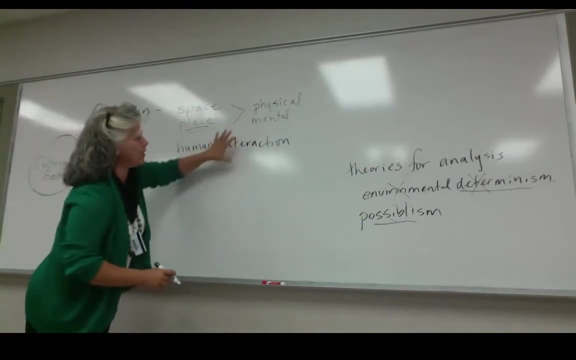 our class Cultural geography. So that's part of this larger term. This is so big. All of these keywords that I have written here go into a good and thorough definition of geography. It's really too big to include in one semester's worth of introductory class. 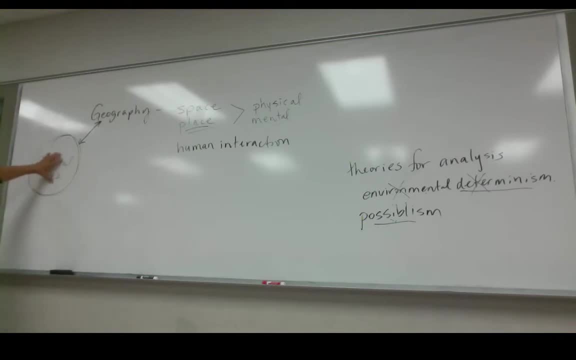 And so we have part of it cultural geography, which we're going to do over here and that's our class. And we have another class you can take. It is physical geography And that looks more at processes in the earth, It looks at weather patterns, It looks. 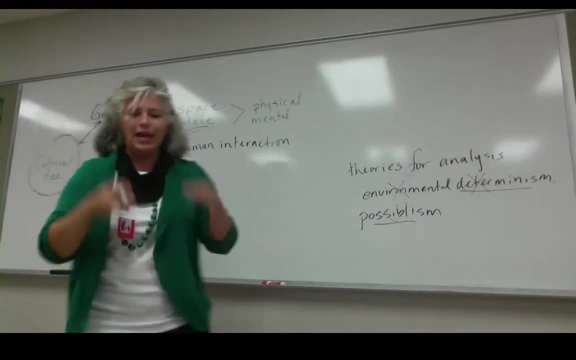 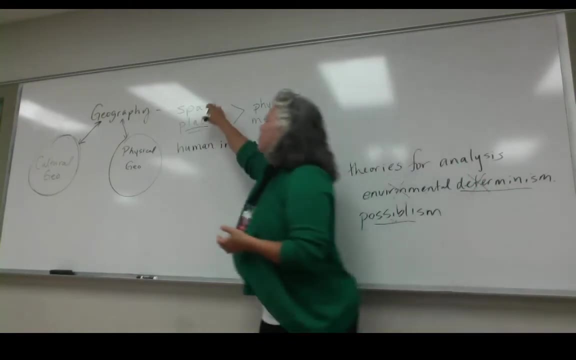 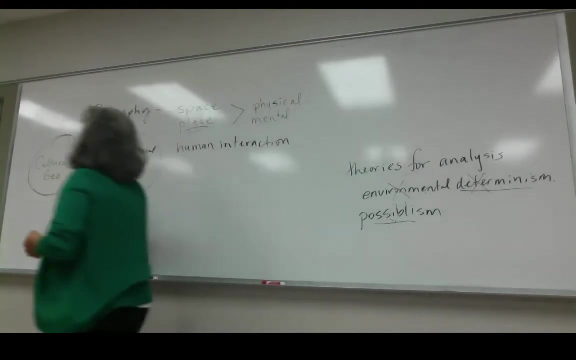 at topography and all kinds of interior physical and atmospheric physical aspects of a place and space. It has place and space in there also, but it's more of the physical stuff And there's a relationship between these two things And so truly. 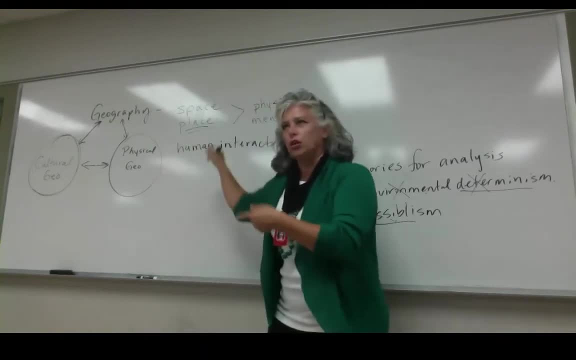 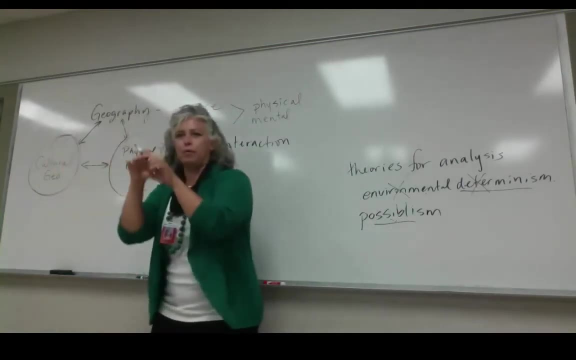 if I had thought out this flow chart a little better before I drew it on the board, really these two bubbles would cross in the middle, They would overlap in the middle, because we can't talk about what people do with their environment without understanding the environment. 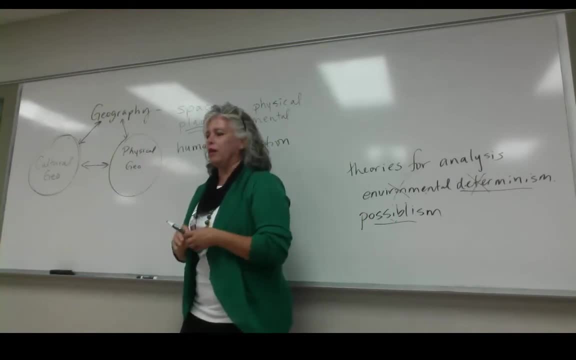 We're just not going to focus on things. like you know. we're not going to have a unit on plate tectonics, for instance. Y'all know what plate tectonics is- Like earthquakes and volcanism and stuff like this- But does 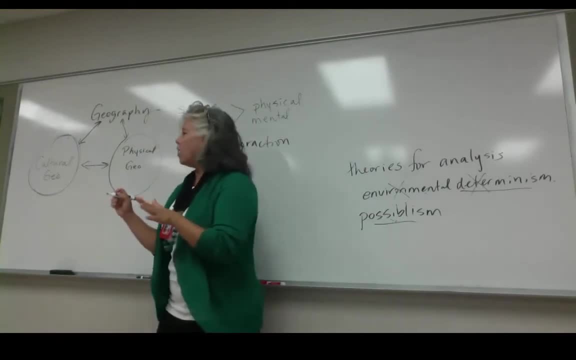 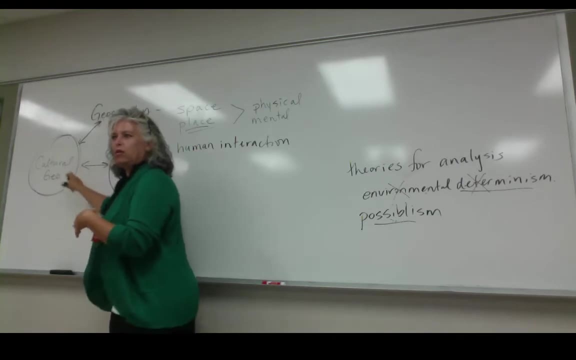 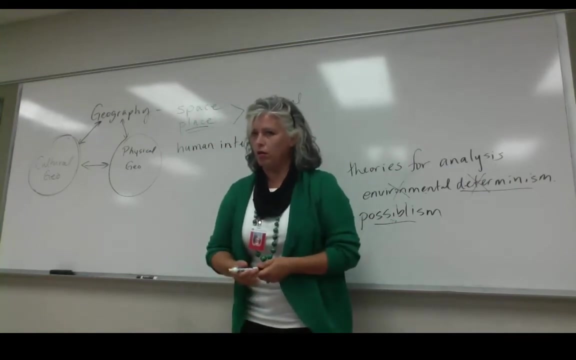 plate tectonics affect. anybody know whether plate tectonics affects the way people live their lives and design their environment? Anybody know Like how Well, I mean like certain buildings cannot be built tall in certain places so you wouldn't see big buildings. 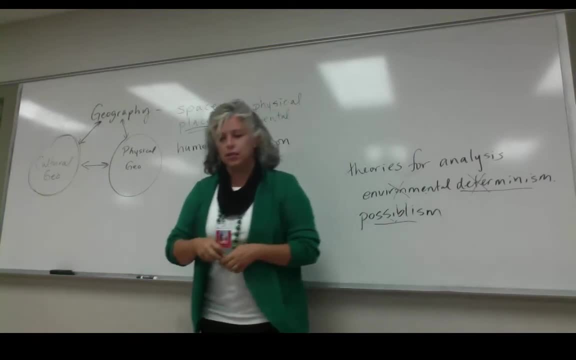 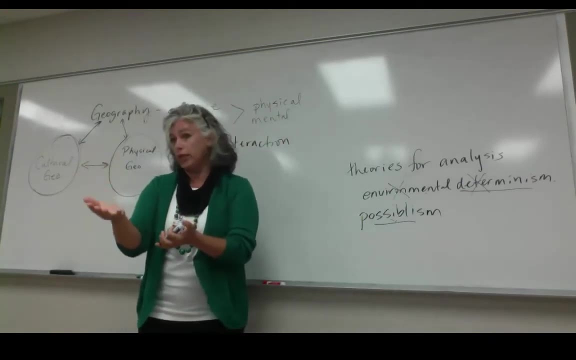 like you see in New York and stuff in places where- Okay, so I don't know if your voice came over on the recording, So yeah, so you're talking about sky scraper buildings, the numbers of stories, So a place like New York City. if we look at the, 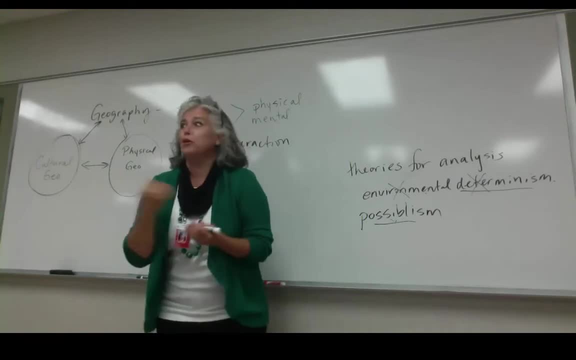 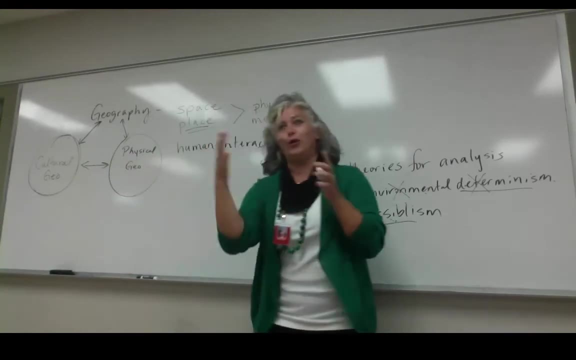 skyline and we see all that. it would be good to assume. I really don't know whether there's a plate boundary anywhere close to New York City. I don't know whether ever in geologic time there's been a huge earthquake there and they have the. 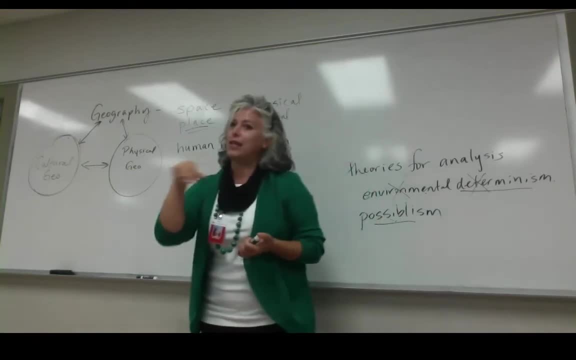 potential of having it happen again. But if you look at the landscape of New York City you would assume no, because there are rules about earthquake. safe buildings, earthquake- I don't know that there's an earthquake proof building. Somebody might know that, Some of you. 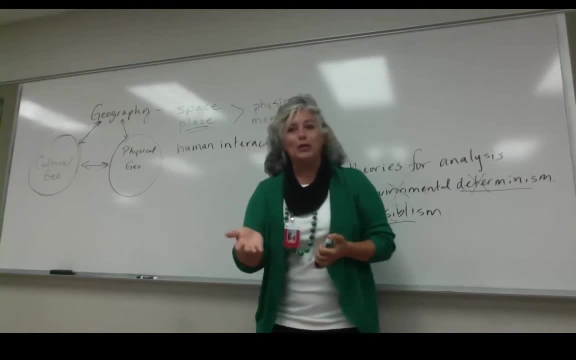 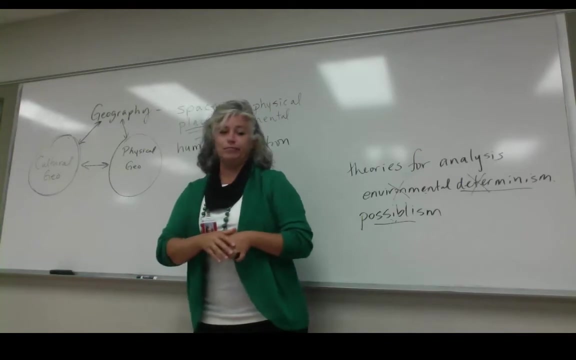 might know that, But there are rules about building. What materials do you use? How high do you build in an earthquake zone? Yeah, because it's going to affect whether your life and property are like survive an earthquake. right, There's also habits. 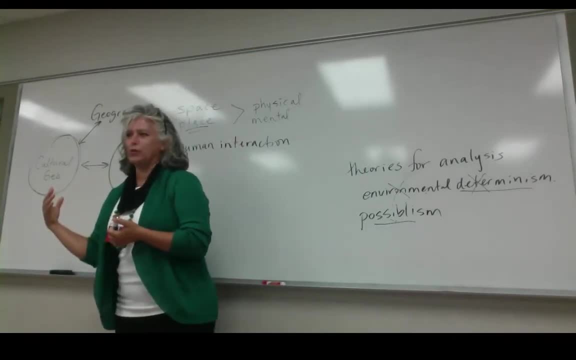 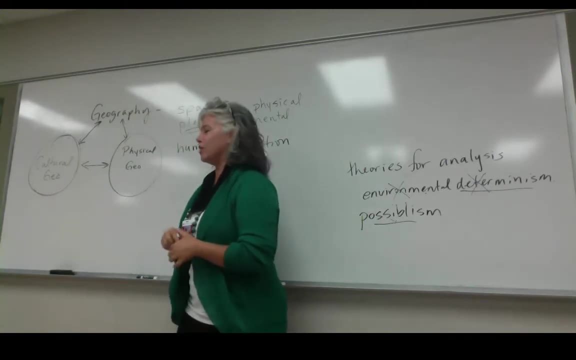 that people- any of y'all ever been in an earthquake or lived at a place where you had to know about? I have some really good friends who live in Costa Rica. I've spent a lot of summers with them, back when I was doing anthropological field work especially. 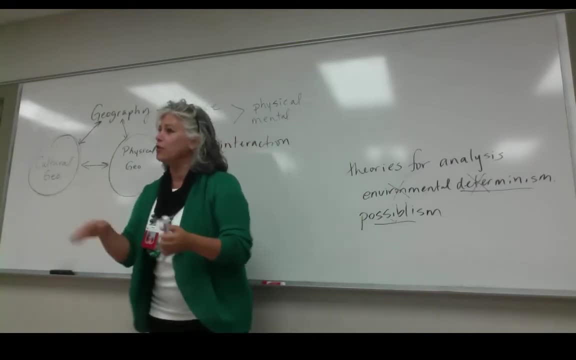 and they have earthquakes all the time, Just little bitty ones, but you can feel them, Like you would be able to feel. you know the projector would wobble or something would wobble, and all of them in their daily life, their habits. 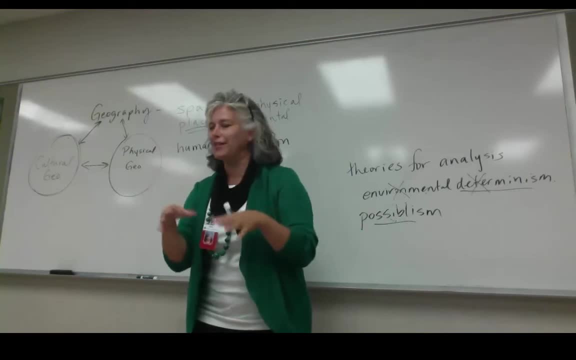 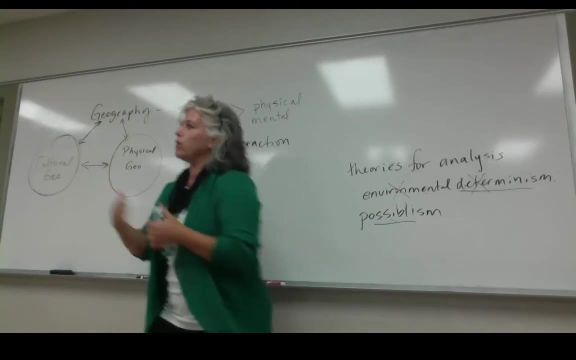 their behaviors when they feel that that tumbler, as they call it, or rumbla, when they feel that they run outside- Oh, it's an earthquake, Let's run outside. They drop what they're doing, They run outside Well. 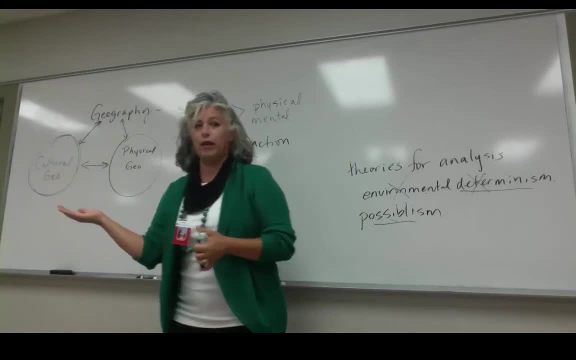 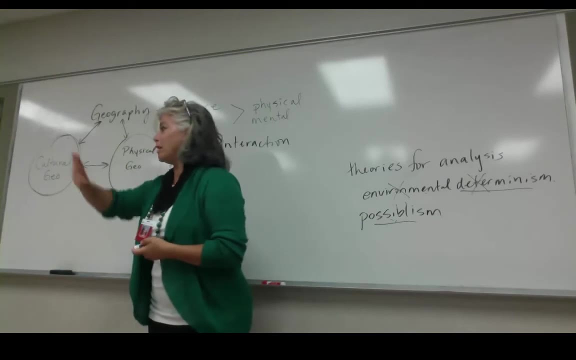 that's something that you learn in a place where there's earthquakes, often because you don't want something to fall. If it's a big one, maybe your walls will crumble, Maybe something will fall on you. Maybe it's safer to be outside, where walls can't. 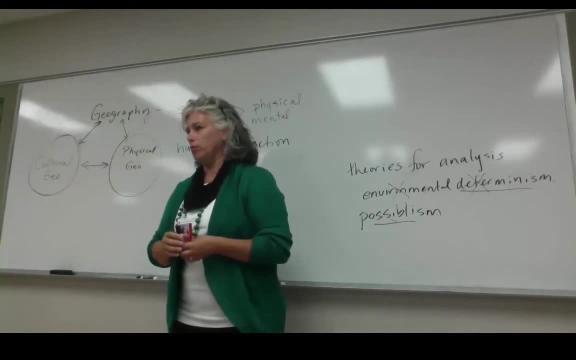 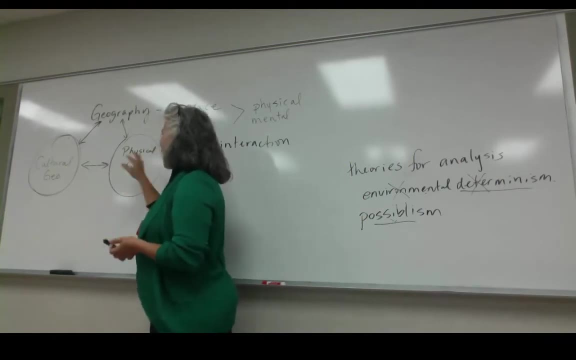 fall on you. Pictures and furniture and stuff like this can't fall on you, And so they make this habit run outside. So that's just one quick example of how we can't forget about this entirely. even though our class is called this, We can't forget about. 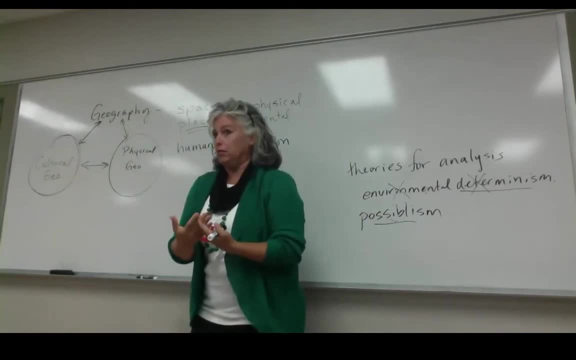 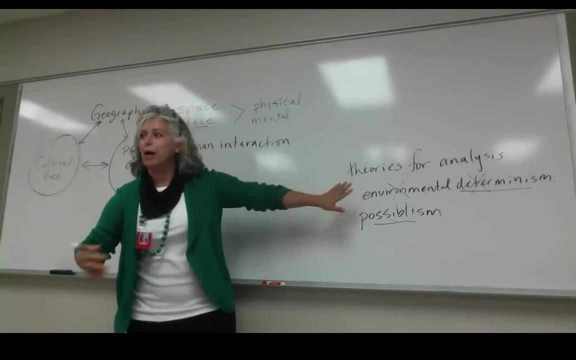 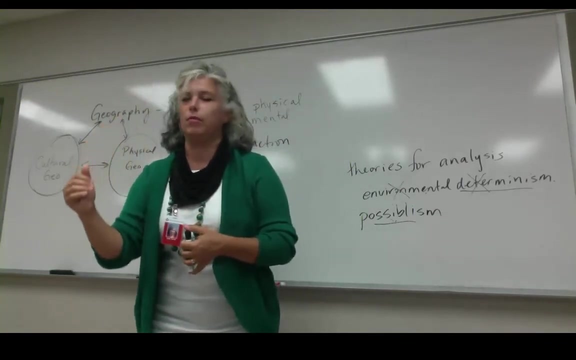 this entirely because they are related. Environmental determinism is not perfect, but it's still valid in some cases. But it's possible to build buildings, even a certain number of floors on the buildings, maybe not a skyscraper, that's 100 stories high. 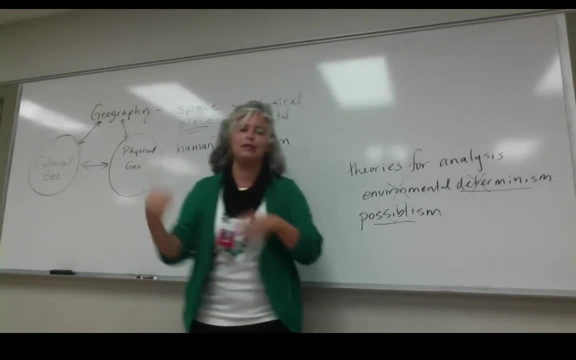 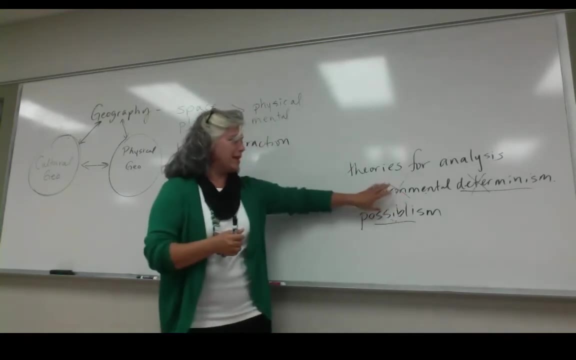 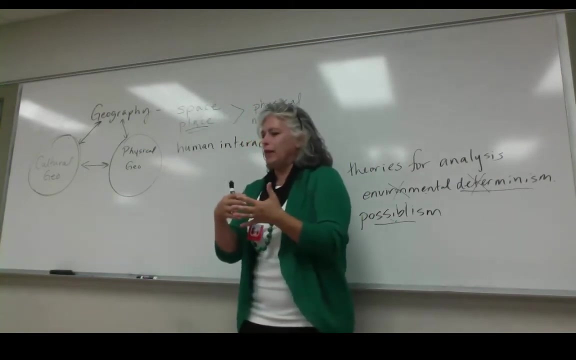 but it's possible to build buildings that have the least amount of impact and problems with earthquakes. So there's like a crossover in some of these theories for analysis. There's like a crossover that we need to be able to use to understand things fully. 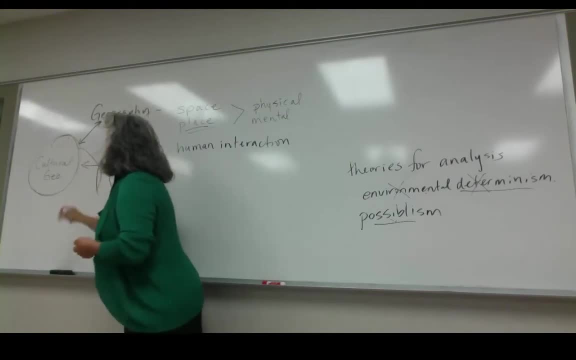 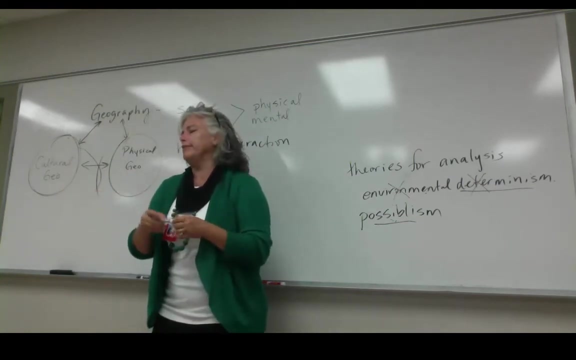 and there's- technically I should have made these bubbles crossover or something like that, because you have to have some kind of understanding, basic understanding of the physical environment, to really fully understand the culture that comes up around or that evolves. evolves means changes over time in 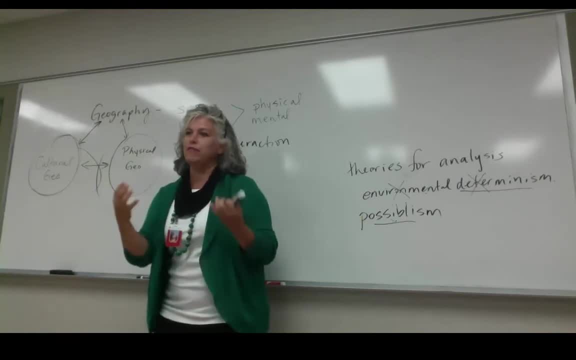 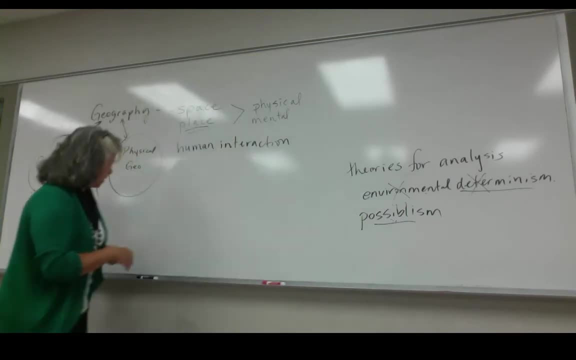 a place in space, in our minds, in the physical sense, when we interact. You got it Okay. Questions while I'm erasing No, Okay, How much time do we have left? 20 minutes, Okay, So let me. 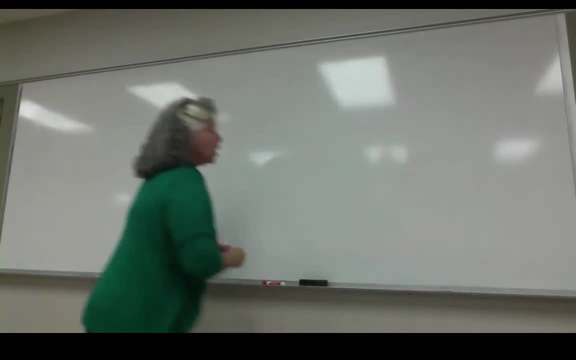 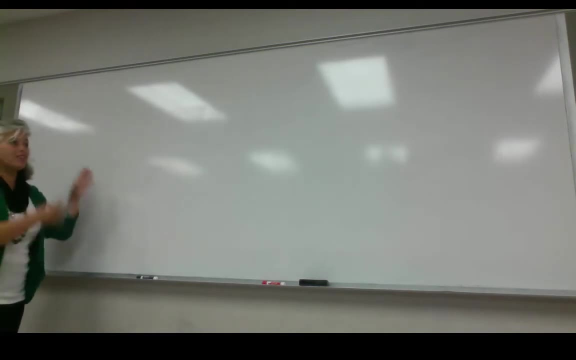 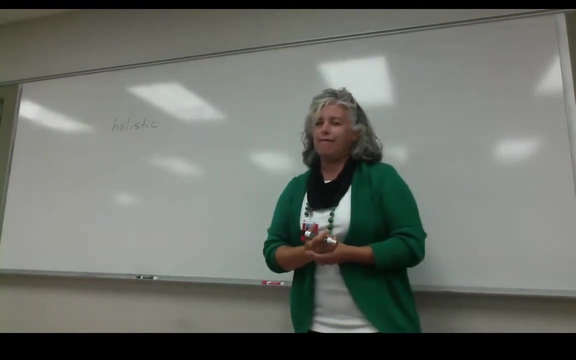 do two things. We will do two things. Let me first say that geography in general, and even when you break it down into physical and cultural geography, geography is something that we call holistic. It is holistic And essentially a very short definition of what holistic. 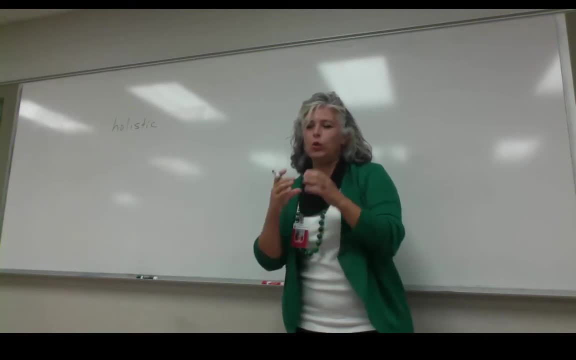 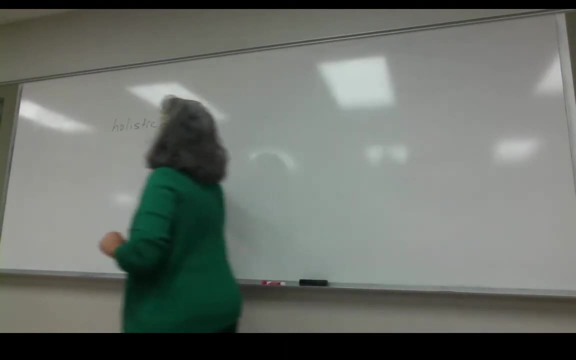 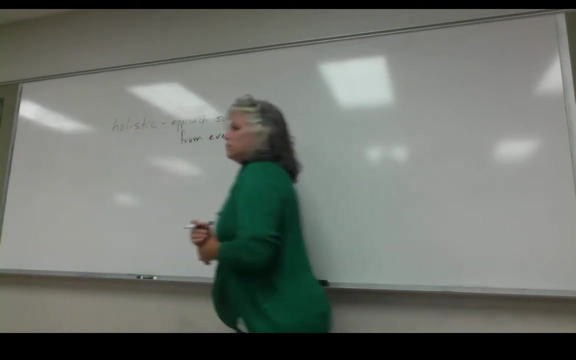 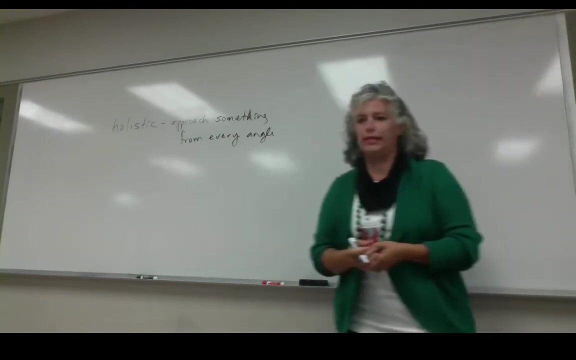 means is that it comes at. if there is a holistic discipline like geography, you come at something from every possible angle, You approach something from every angle, And that's a very short, little quick definition of holism or holistic. Siri will give us a better one. Let me see. 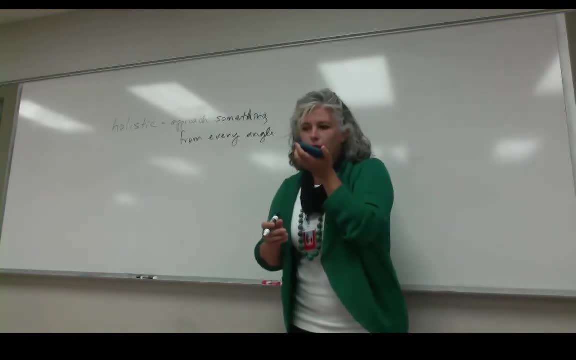 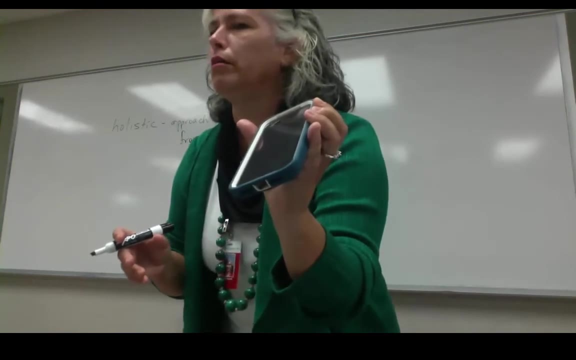 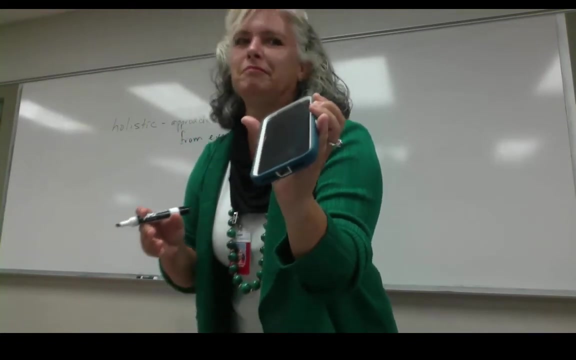 if Siri will give us a better one. Siri, what does holism mean? Holism means the theory that parts of a whole are an intimate interconnection, such that they cannot exist independently of the whole or cannot be understood without reference to the whole, which is 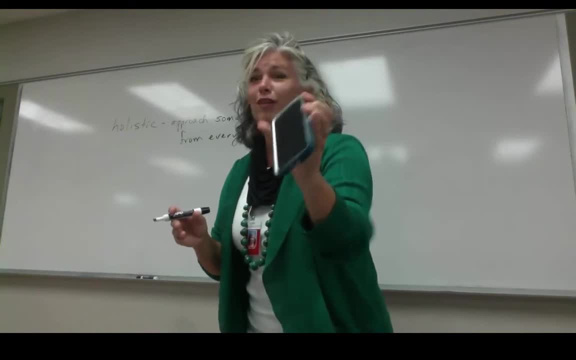 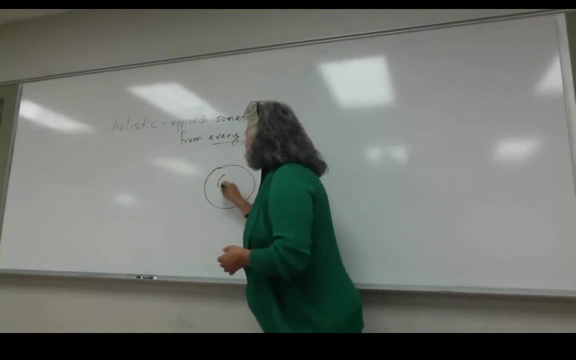 thus regarded as greater than the sum of its parts. Too much, Too much, Right, Okay? So holism means you try to understand something from every angle. So if I have that circle with geography in the middle of it here, right, Geography. 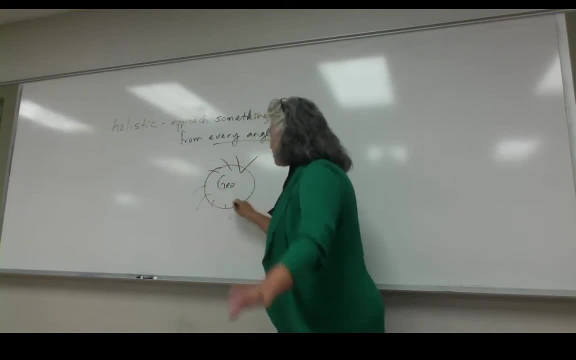 There are so many little to use some of. what Is that? Looks like a really ugly germ molecule, doesn't it? But anyway, or whatever looks like a germ. Anyway, all of these little things coming out, they would be history and math and science. 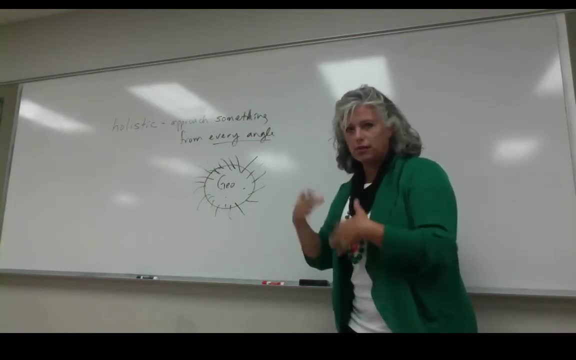 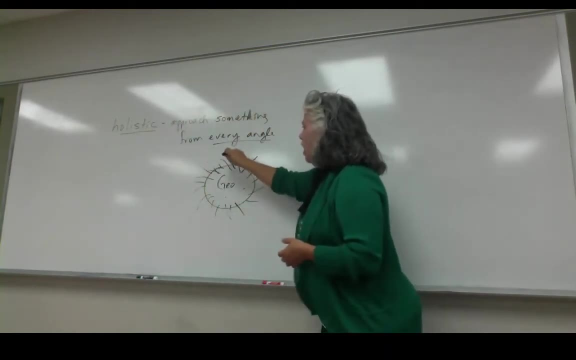 and music and philosophy and art and etc. etc. Like put everything, If you want holism to apply to geography, then you've got all of these little tentacle kind of things that branch out into architecture, winemaking, clothing patterns. 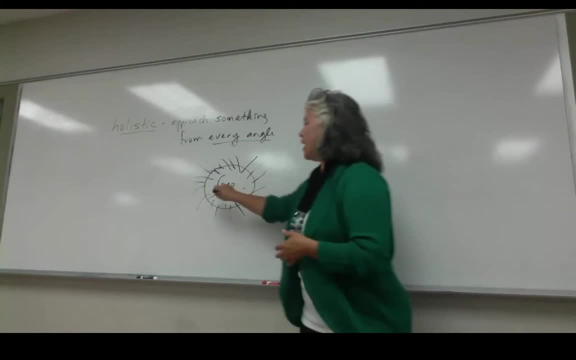 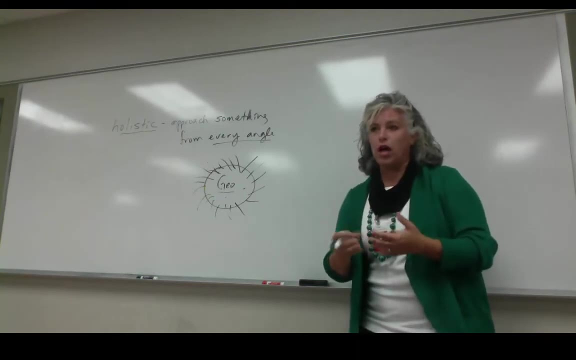 musical forms. All of these things have some kind of relationship and contribution to really fully understanding the way a geographer thinks about and classifies the world. Okay, So geography is holistic and so, even though geo literally means the earth and geography draws or sketching the earth, 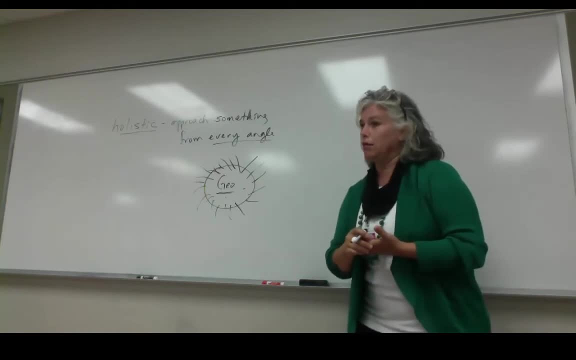 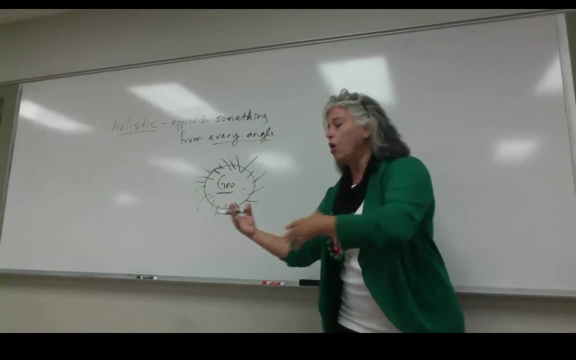 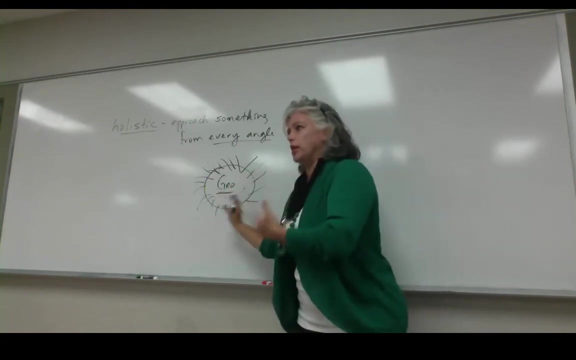 we can talk about a moon colony and how things might be possible to carry on human culture on a moon colony where the environment is really different. So we can talk about astronomy. we can talk about Scientology and other religions. we can talk about all of these. 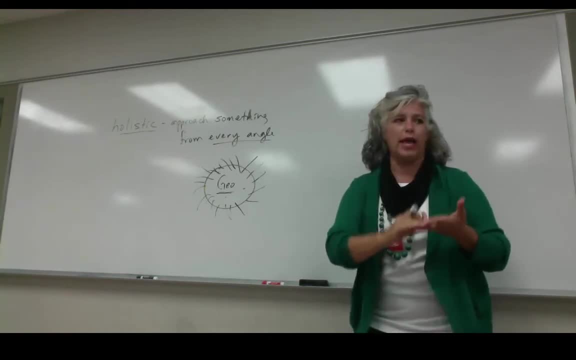 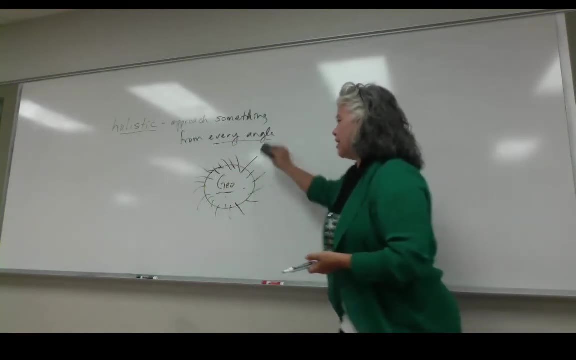 things as affecting our space, our place, our physical and mental mindscapes. Okay, So geography is. Geography is holistic. This is really ugly. Let me erase it. I wish I could draw. I think my classes would be so much better. 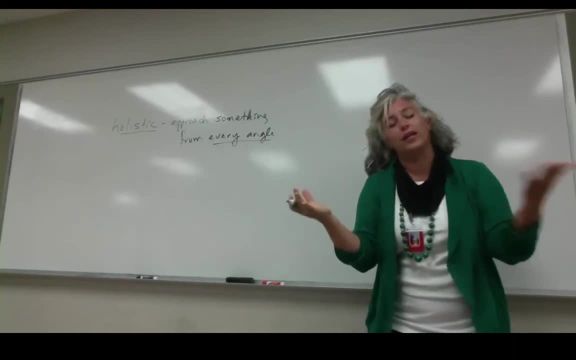 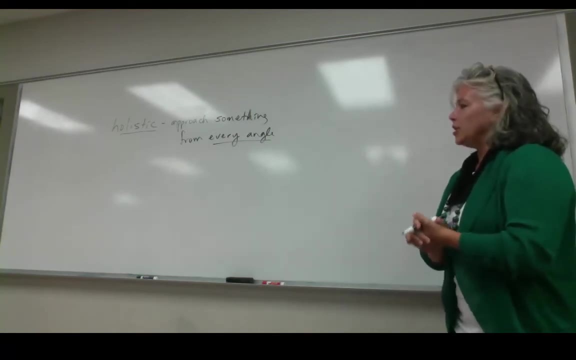 if I could do like caricatures and stuff. but oh well, you, Sorry, You've got me Not a. I don't even write beautifully Anyway. So geography is holistic. So don't use series definition. Use the one that we have here. 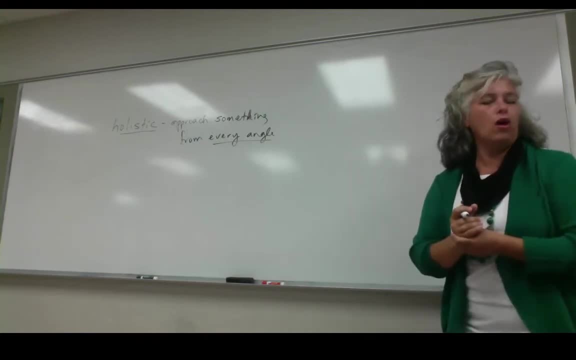 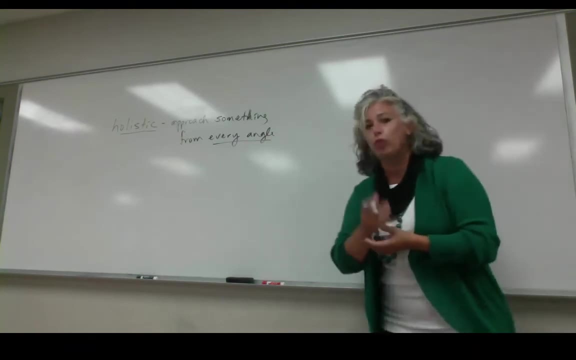 You want to approach an understanding of something from every possible angle. So, if you are interested in music, if you're interested in video games, if you are interested in food, if you're interested in whatever, that's one of the approaches that you can. 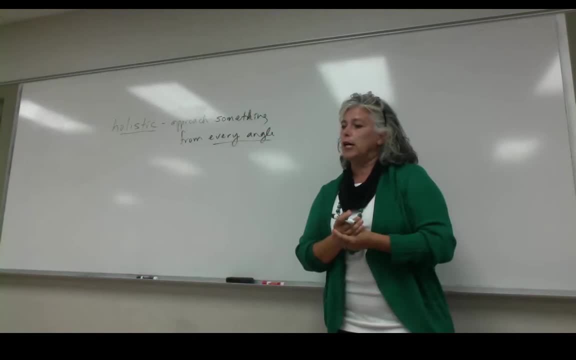 use to understand geography The very first. You know we have five little projects that you all do in here. there's not five, there's four. Pardon me, Nobody freak out. There's four projects that we do in here, 50 points each. we do them with each unit. 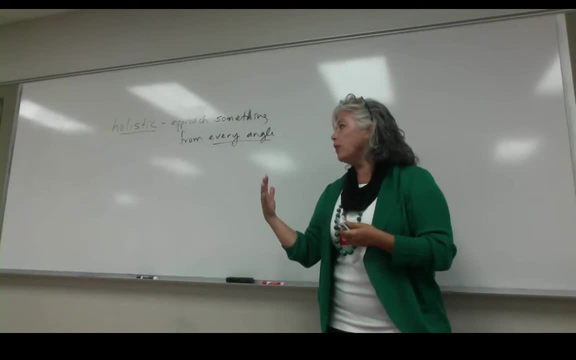 The very first project that we're going to do has to do with some topics that I'll cover for you on Friday in a different video and and next week also, but you're going to be able to choose an area that interests you. I'll give you some suggestions too. 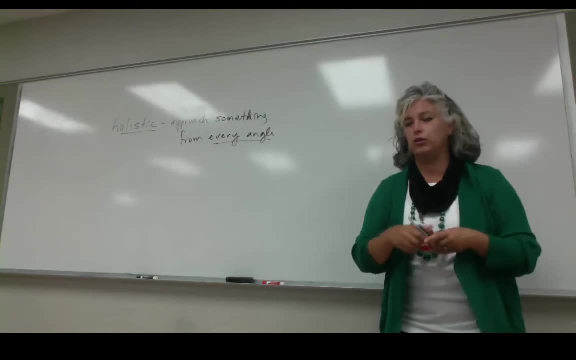 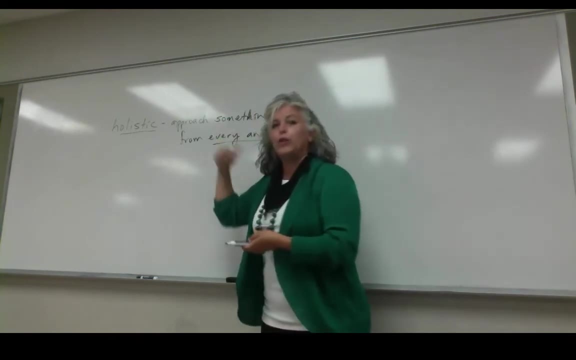 I'll give you some movie and TV ideas and you can choose your own if you would rather, but you're going to be able to choose an approach that you want to take to answer the questions that I have for you on the very first project that we're. 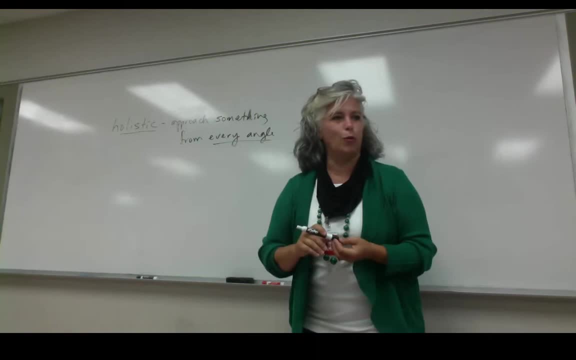 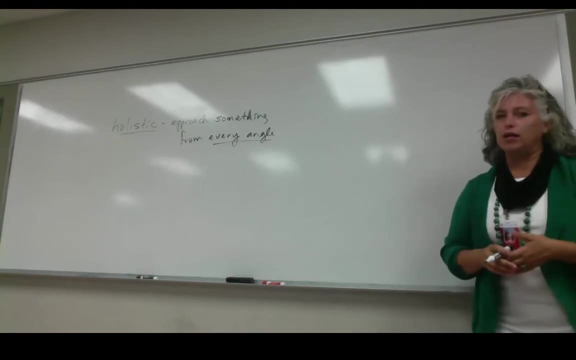 gonna do in like three weeks, I think. it's when we're we're gonna assign that and get a get a due date. but from this day, day one, note-taking day one- we're getting that information, we're building that information that you're gonna need to ace that project and to to do well. and so holism is a concept that is a big 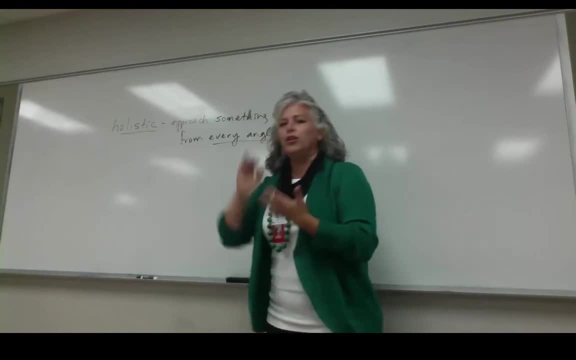 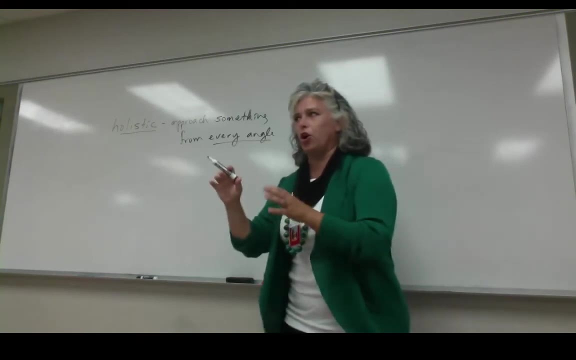 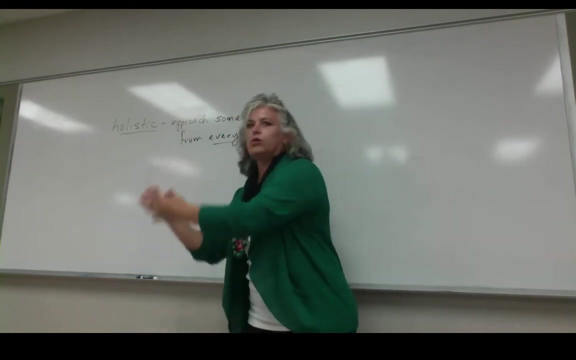 deal because not every you know. you take a psychology class and that's not holistic. it does not look, for instance, always there are aspects of psychology that you can look at- a social environment and how it affects people, but that's the realm of sociology. how do people interact in their social environment? right, you can. 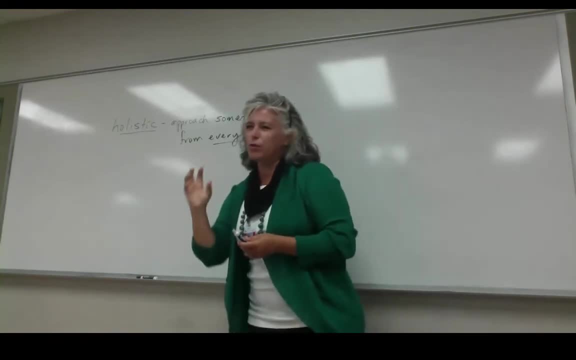 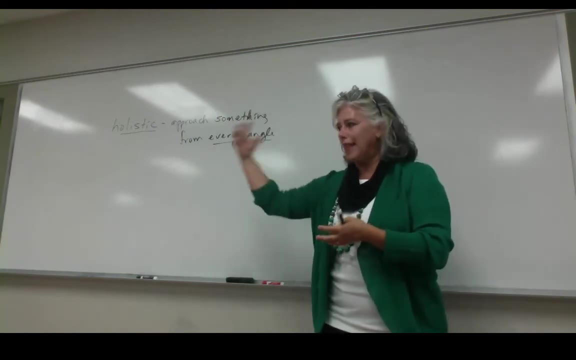 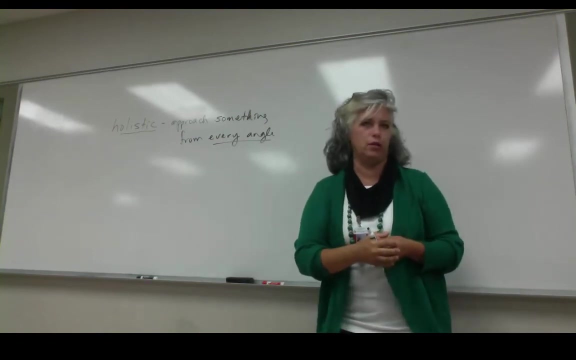 go to biology and there's certain aspects of chemistry that work in your anatomy and your physiology, but you don't focus on chemistry or look at that discipline in conjunction with biology. all the time it's like one unit. you don't focus on chemistry. all the time it's like one unit. 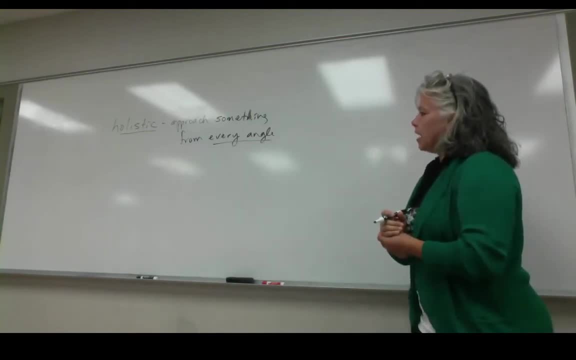 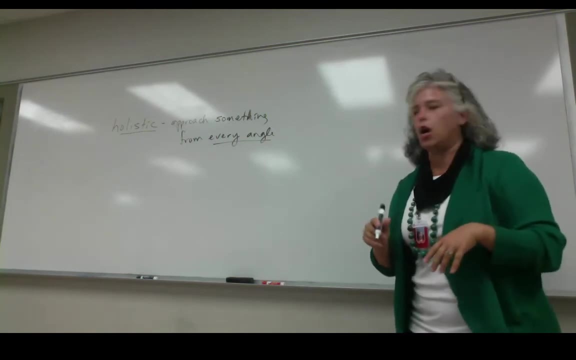 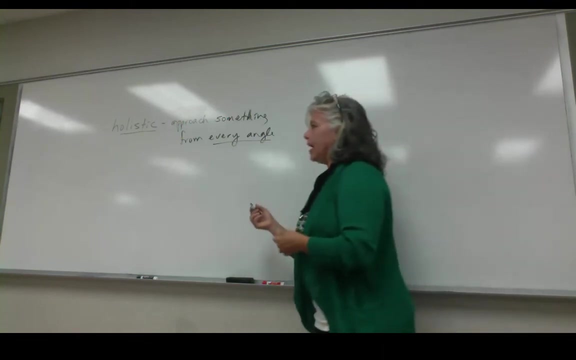 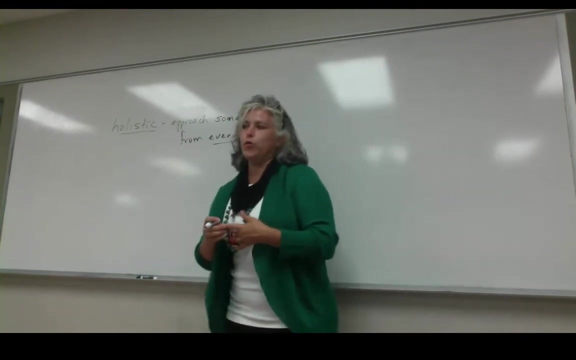 right. so holism is something that we're going to come back to because, if you're interested in it, it's geography. we can make it relate to geography, okay, so the last thing I want to have in this lesson for you today is thinking geographically. one thing I've noticed over the years is my students and you don't have to- 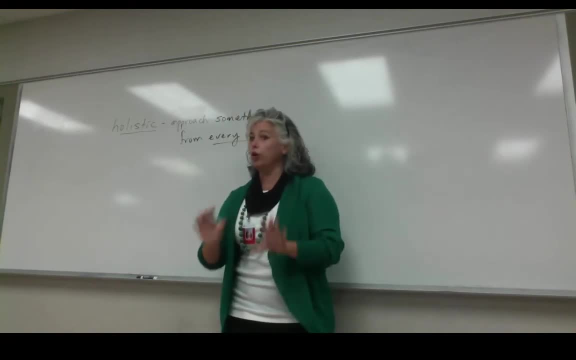 confess if this is you, but my students are really good, y'all are really good at thinking from the mindset of a historian. what does a historian really? what are the questions that a historian usually asks? just the basic questions, and what I'm talking about are the question words like 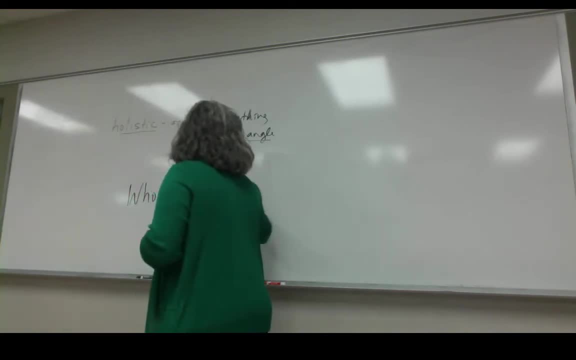 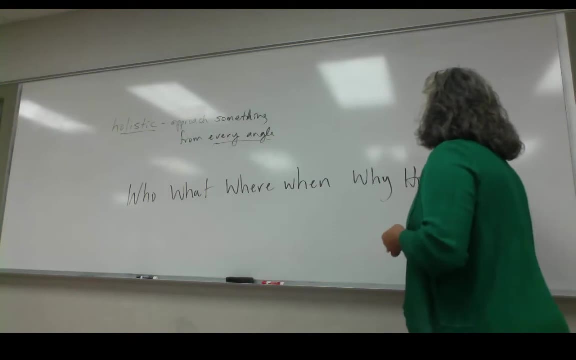 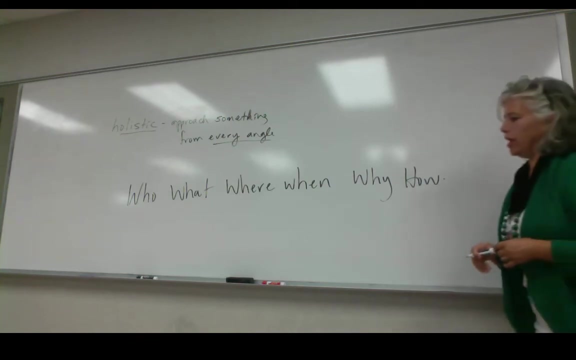 who, what, where, when, why and how. I'm going to start with this question of who, what, where, when, why and how, why and how. These basic questions, Which ones of these do you think stick out to you? 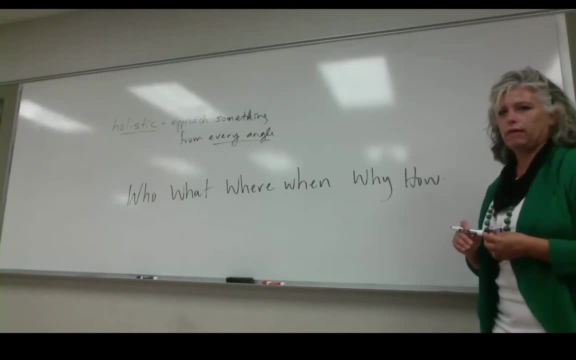 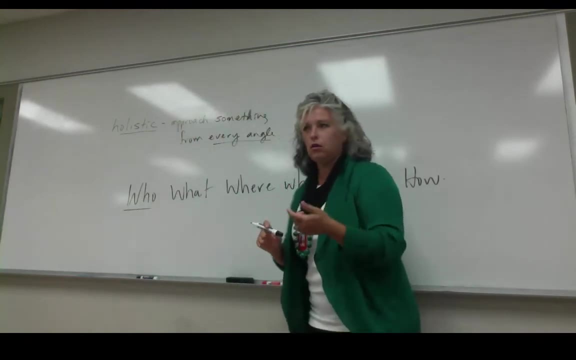 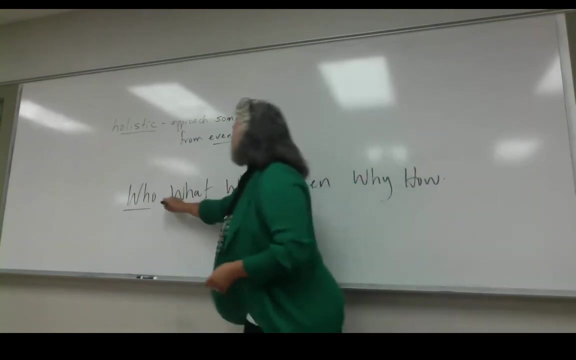 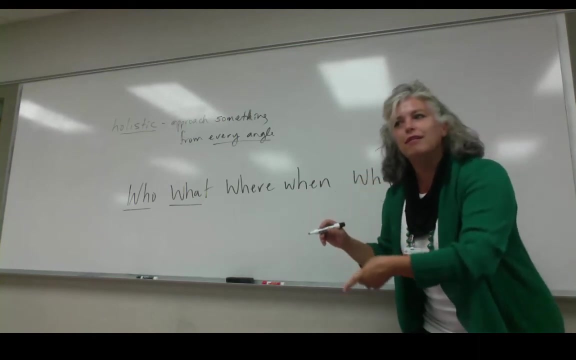 as history words. You think who is a history word? Y'all agree. We want to know who. Who did what? Okay, So is what a history word In history? you want to know who did. what Are dates really important to historians, Who did what when Right And when you get? 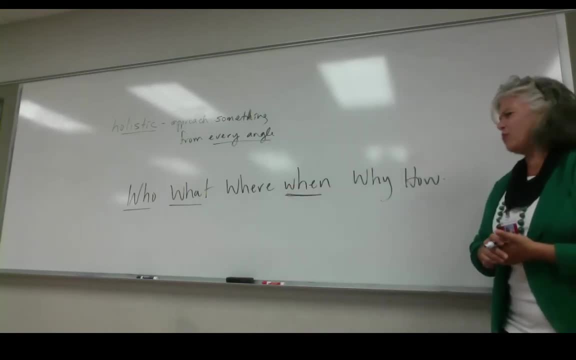 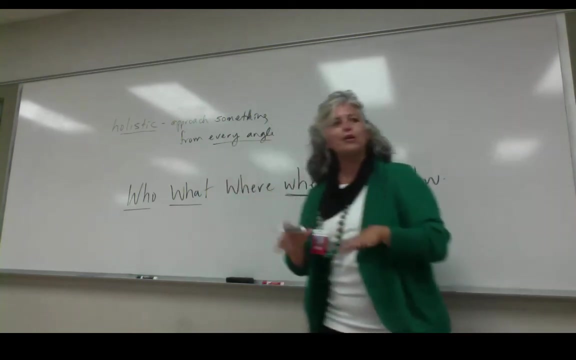 more complicated into history. it's not just memorizing who did what when It really isn't. It's really understanding more deeply why and how something happened And sometimes where matters Sometimes, But the main things, especially in the early classes that you take in history- 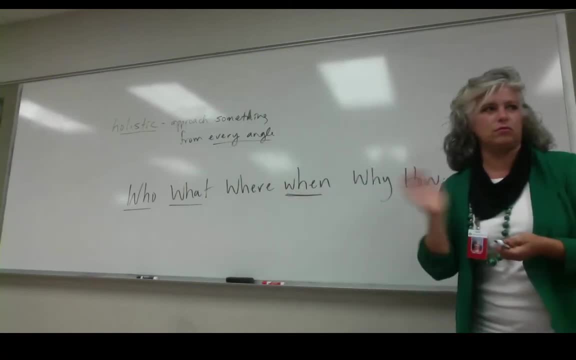 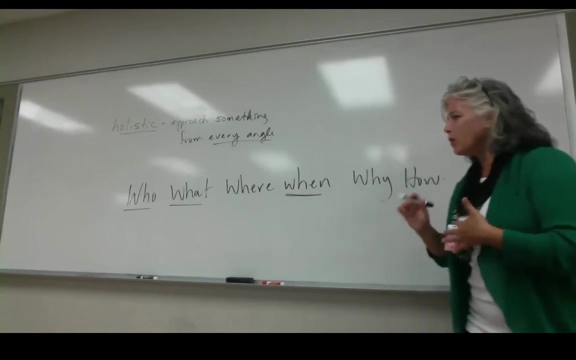 are who, what and when. Right, You agree. Okay, I'm getting some agreement. Okay, In geography we are really different. It's not that we don't care who what when, We don't, But was: who, what, when? can you relate any of these three words to those key words in? 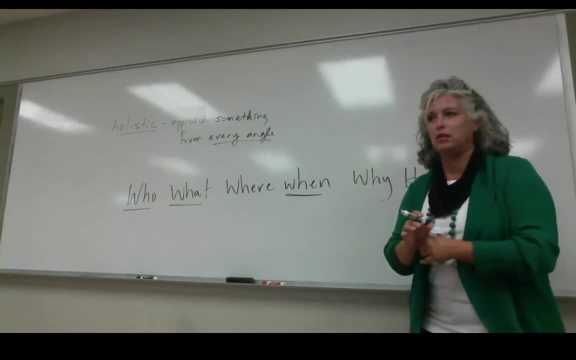 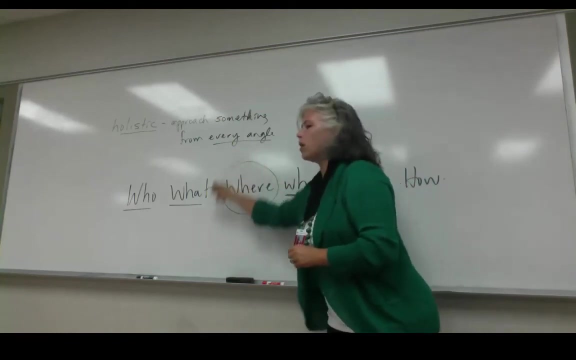 the geography, Like place and space and mind and physical. Like you can't easily relate the who, what, when to those key terms in what geography is, But you can, because place and space are there. Here's a geography word And the main question that we ask in geography, the holistic, 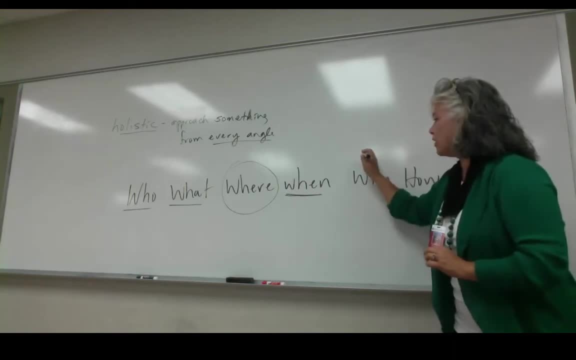 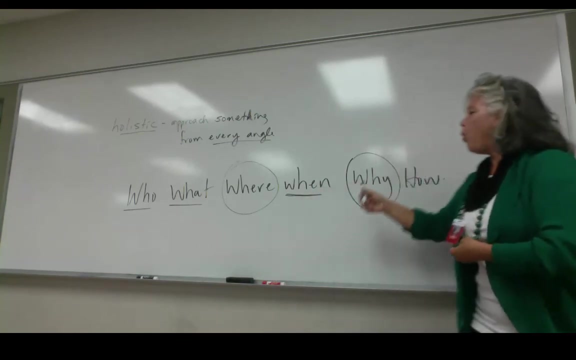 discipline of geography. the main question that we want to know is why, where something happened, The why of where something is happening did happen, probably will happen. Why did something change where it transitioned to, for instance? So I was telling y'all earlier. 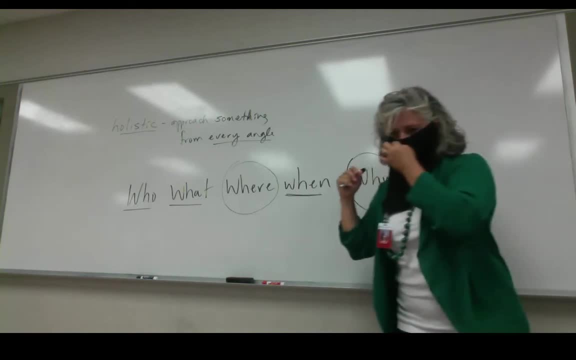 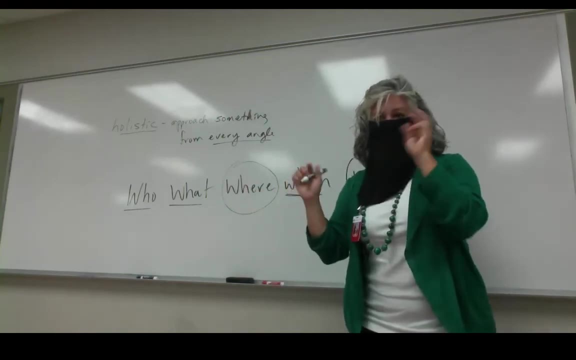 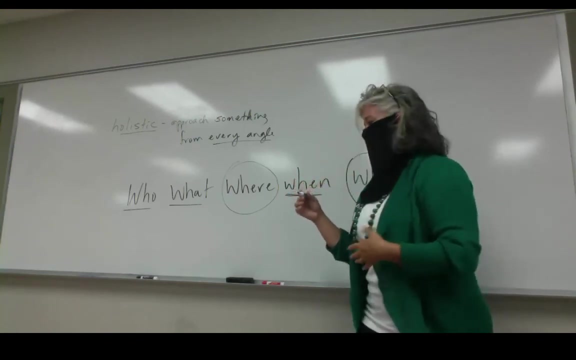 this is my mask that I have. I have a whole bunch of these in different colors, because they were like $2.99 on eBay. So this is not a mask designed for the purpose of protecting us from the disease antigen that we're trying to get protected from. This is a religious article of. 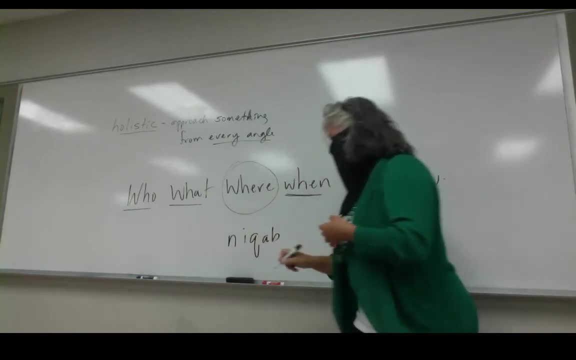 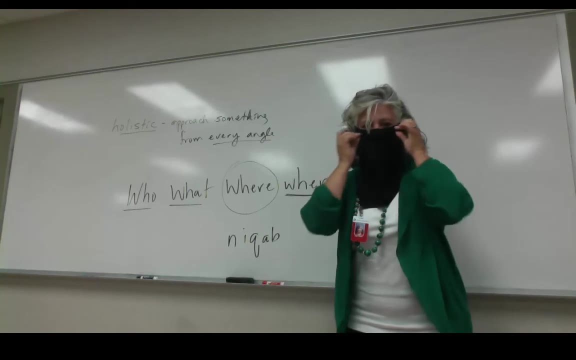 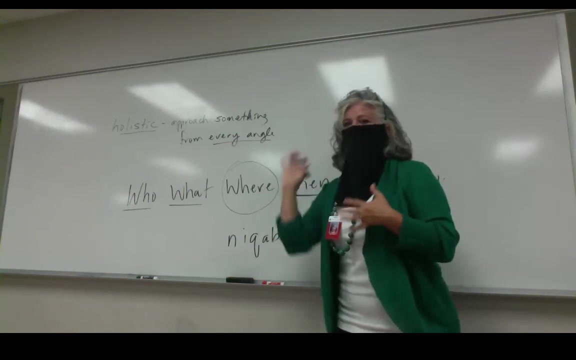 clothing called a niqab. Y'all can search for them on eBay. They're $2.99 each. This is a religious article for modesty that Muslim women wear, Particularly in Asia- this is a fabric that is used a lot- and the Middle East, because it's really hot in those places, equatorial places. 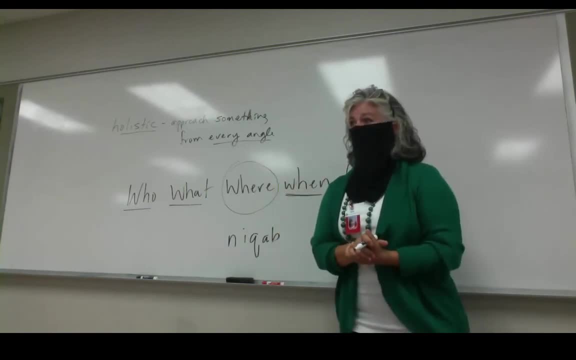 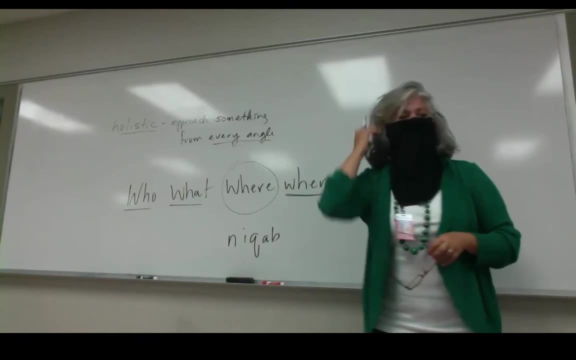 So I bought myself some of these because we need masks right now, And the other little masks I just like you were saying. they fog up your glasses, they fog up mine too and I have to put mine on and they're hard to breathe in. 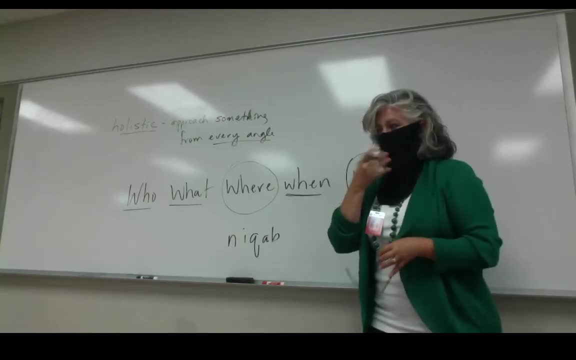 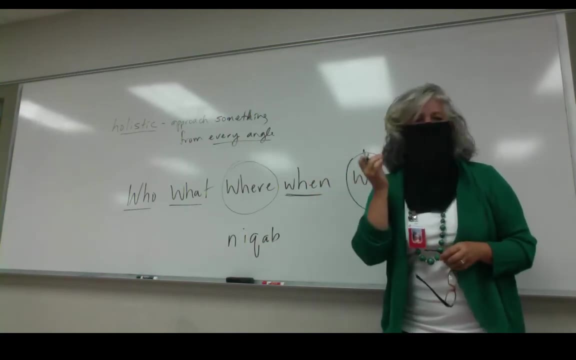 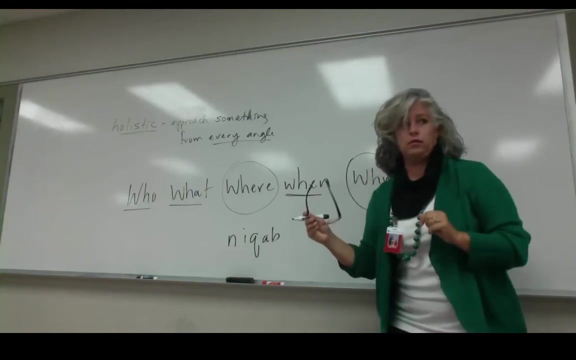 So I bought a whole bunch of these because they are cooler for me to breathe in in this hot summer weather that we have. That's not the purpose for which these were designed. This is not one of the cloth masks that you can get at Walgreens, because originally it's for that religious function of 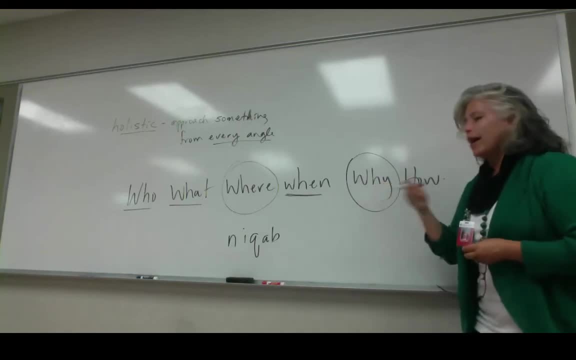 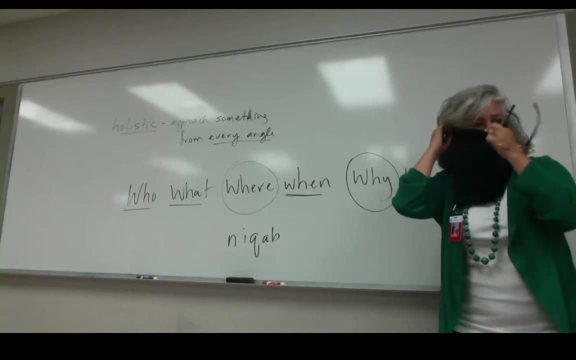 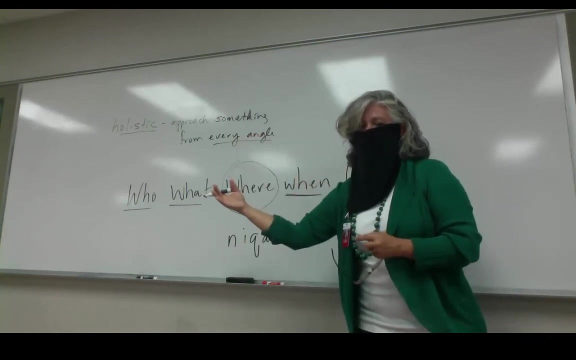 modesty. But why am I using it where I'm using it? where Muslim women? you know Muslim women are not common here in central Arkansas- Muslim, you know. I can't go into Target and find a turnstile with these on it in the clothing section right. 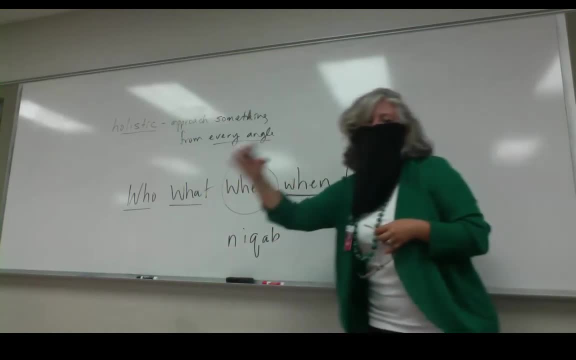 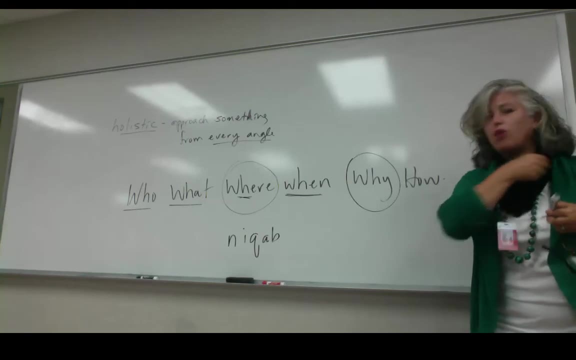 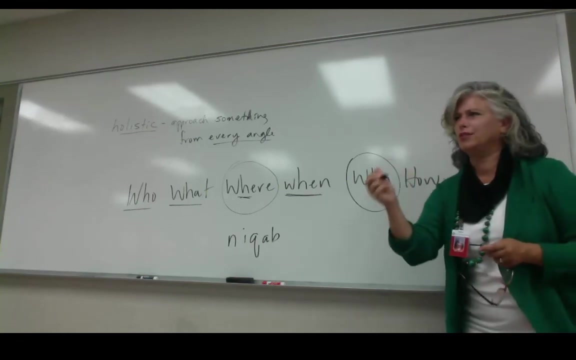 So why do things change their purpose when they diffuse to other places? So this, the purpose for which I'm wearing this, is not religious, it's not modesty, it's the disease: antigen or contagion- pardon me, antigen's not the right word, contagion. 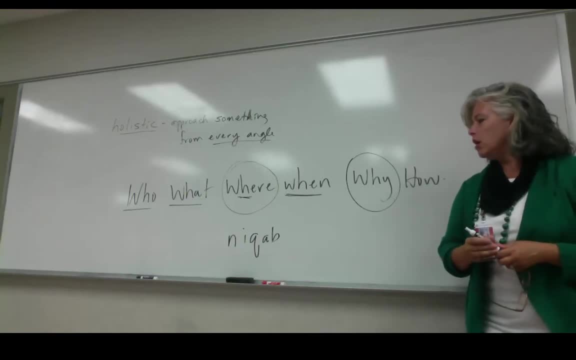 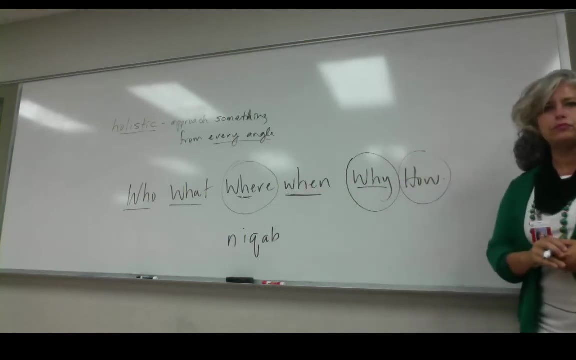 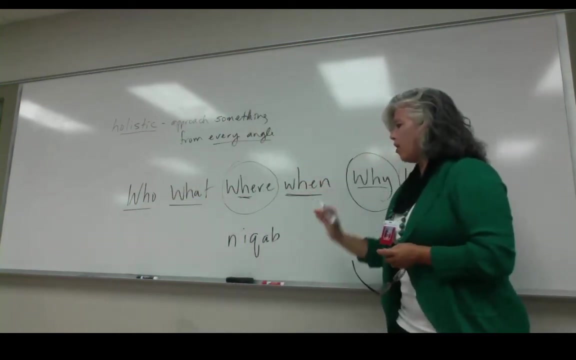 Contagion Is the right word that I should be using here. So in geography, our main questions are why, where and sometimes how, And we might want to get to these things also, but they are the fourth, fifth and sixth things that we get to. 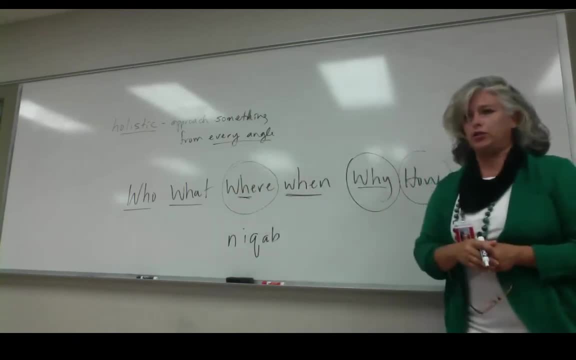 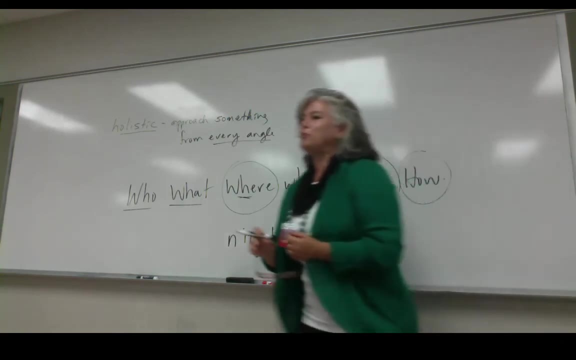 Whereas in history these are the first, second and third things that you get to, and then these are the fourth, fifth and sixth things that you get to. So let's do a 180 with our history conditioning- I guess I'll use that psychology term. 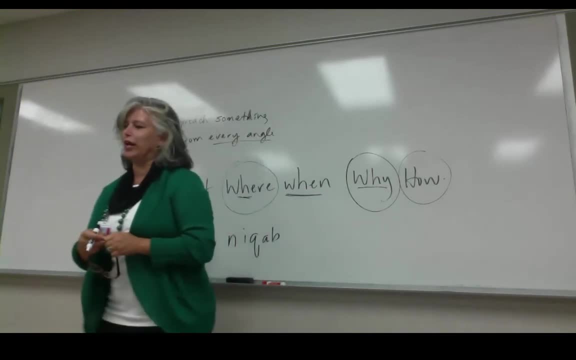 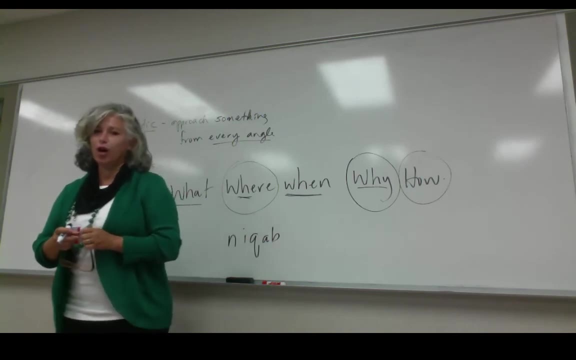 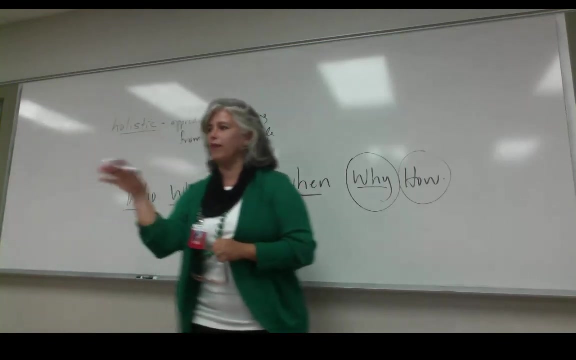 We all seem to be very conditioned about thinking as a historian. we got to practice thinking as a geographer in this class and I'll help you, But that's what we're going to do, for our first project is try to think like a geographer, and on Friday you will have a video posted. so even if you are a face-to-face student with me, you're still going to do virtual, like all the online students, on Friday. 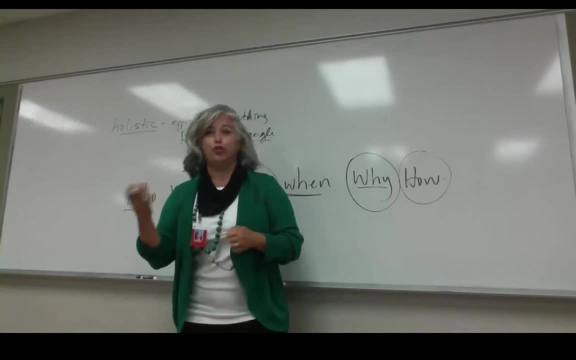 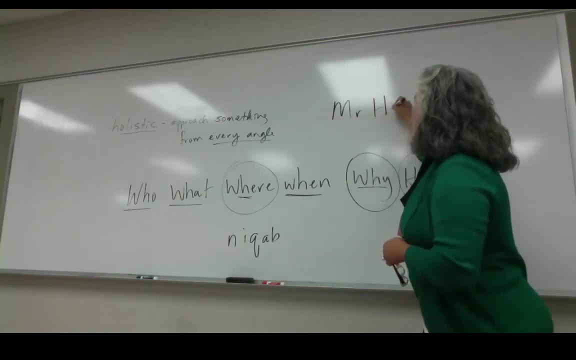 On Friday, I'll post a video that goes over the five major themes of geography. Are we out of time? Well, I'll stop with this. The themes of geography. I won't tell you what these are right now, but there's this acronym: MR HELP. 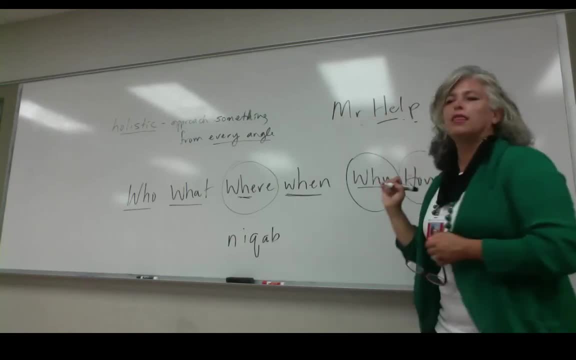 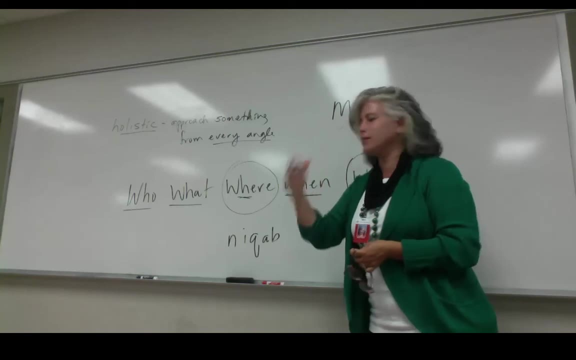 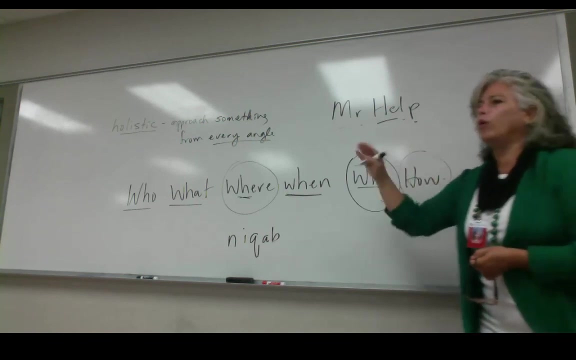 Each of these stands for a different theme of geography. there's five themes, And all of these themes help us reprogram our minds To the where, why and how, questions that are at the forefront of geography, rather than the who, what, when, that's at the forefront of history. 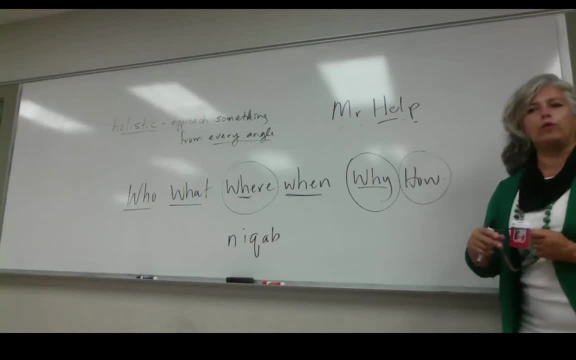 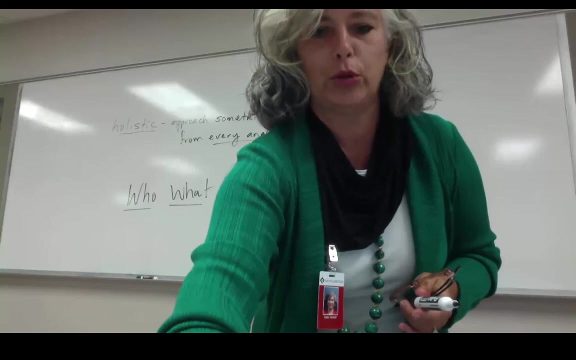 Okay, so that's what our short video on Friday will be about. it'll be about MR HELP And I'll tell you all about our good friend MR HELP on Friday. Any questions? Okay, I hope I didn't speak too quickly for all of you out there on YouTube.